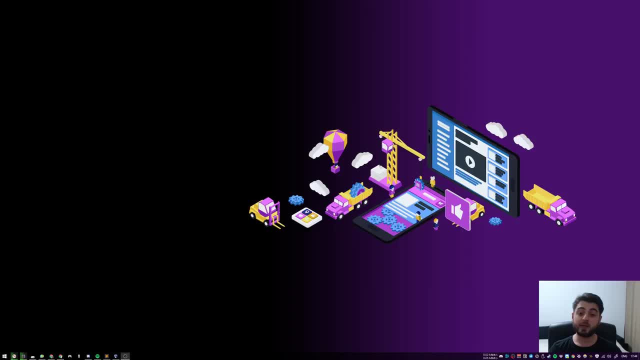 In this video I will simply introduce you to the concept with a few examples, and we might even discuss a few technicalities that surround the topic, But only in the next video you're going to see arguably the most important benefit that you get from them. You will learn about one of the most fundamental techniques in 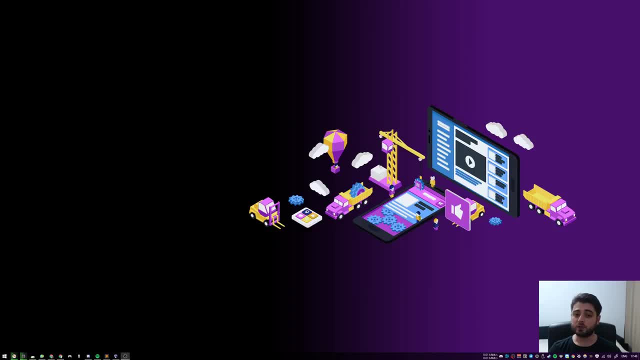 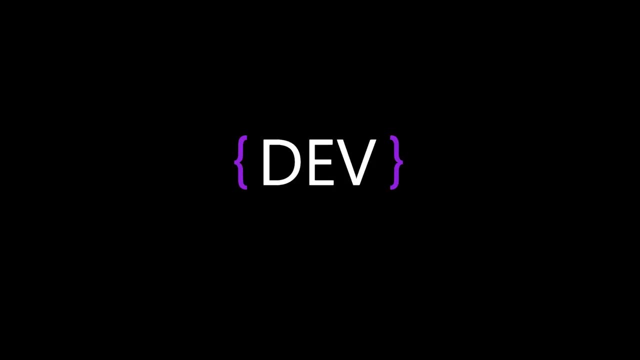 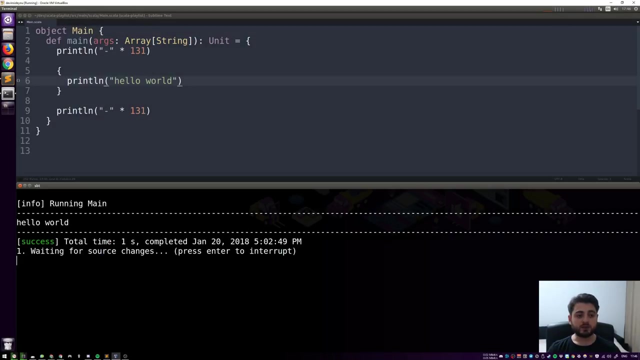 software craftsmanship, You will learn how to harness the power of inversion, of control, which is impossible without higher order functions. As always, we're in the virtual machine which runs Ubuntu and we have Sublime, this time at the top, and the terminal at the bottom which runs our code. This time, before jumping straight, 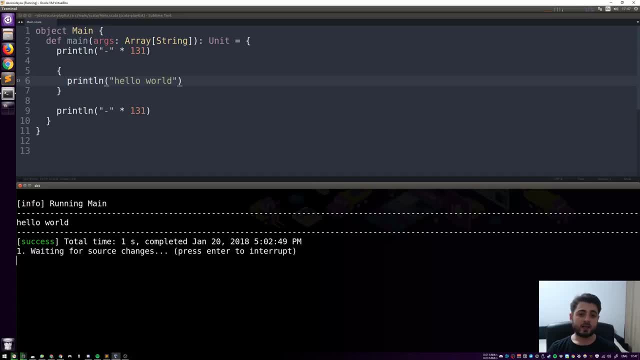 into code. let me say a few things. This playlist is called Scala, your first programming language, for two reasons: Firstly, the actual name doesn't really fit into a YouTube thumbnail and, secondly, I assume that Scala is the first programming language that you get to learn. I'm repeating this because the topic that we're 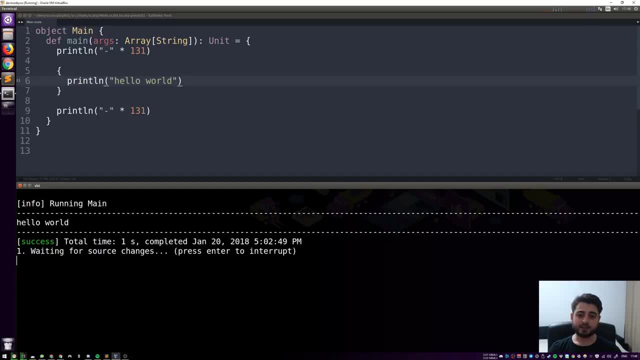 discussing today can be mind-bending for people who are accustomed to other programming languages, specifically languages that don't support the so-called functional programming style very well. Also, remember, in the video about subroutines, we played with functional literals Well. 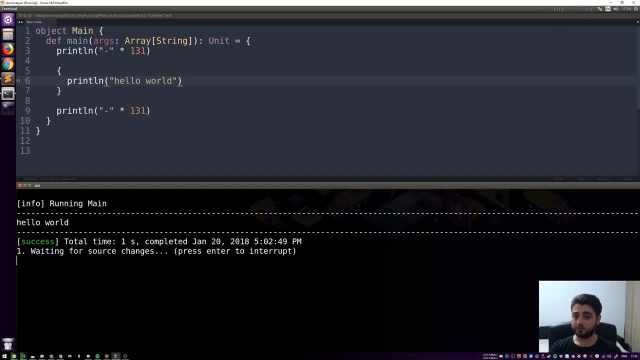 the thing is that even functional literals are not present in every language. If you learn about them a little later, then usually they're introduced to something special, some extra feature from some other world. The word paradigm also gets thrown around a lot. However, if this playlist is, 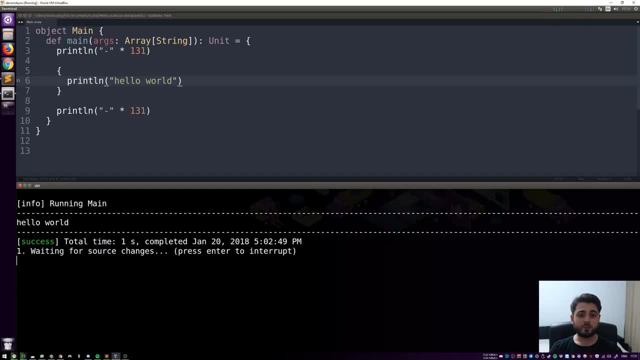 really your first exposure to programming, then I hope that the way I explained functional literals didn't even make you think twice about them. The same way you can use an integer literal to create an integer object out of thin air, exactly the same way you can use a function literal to create 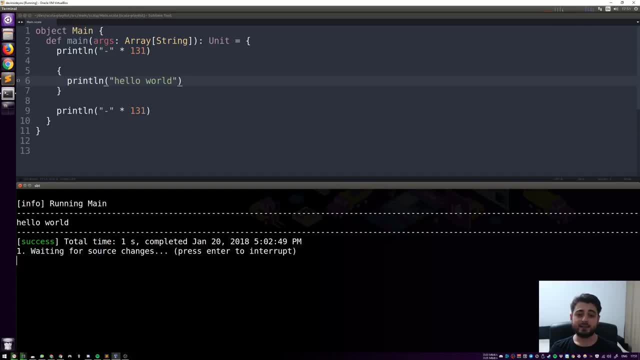 a function object out of thin air, The same way you can bind an integer to an object out of thin air. exactly the same way you can bind an integer object to a variable called favorite number. exactly the same way. you can bind a function object to a variable called favorite function. The same way you. 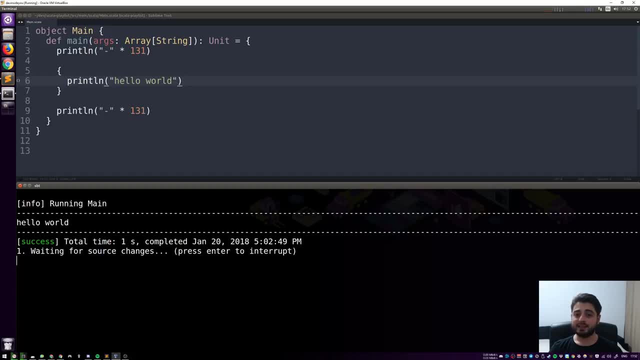 can pass an integer object to a function called show. exactly the same way you can pass a function object to yet another function called show. You get the idea. The last example gives you a taste of what higher order functions really are, Whereas an irregular function accepts and produces instances. 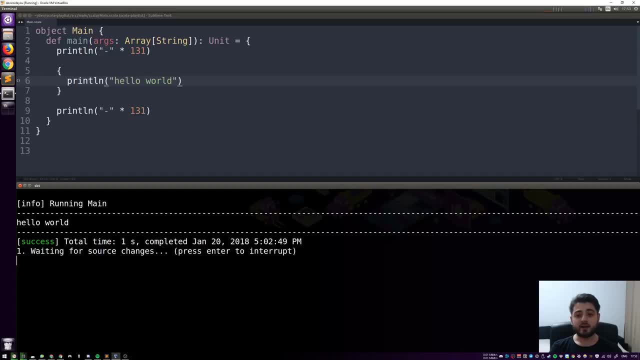 of irregular types like integers, booleans or strings. a higher order function accepts or produces other functions. In this video we'll talk only about the first part- functions that accept other functions as their arguments- and a few videos later we're gonna talk about functions that produce. 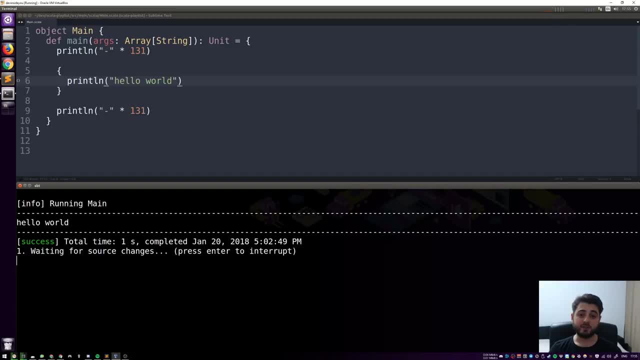 other functions as their result. By the way, the last few minutes in the previous video already talked about this topic, even though I didn't mention it explicitly. I didn't call them higher order functions. Remember this method called left to right, that would accept the left function and the 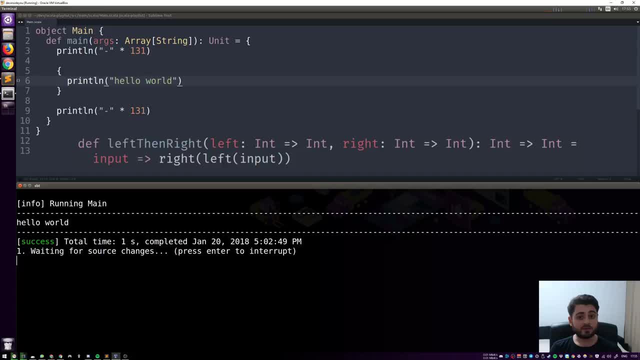 right function and produce yet another function. That was a higher order function. Or remember when we were saying 1 to 10 for each print line? Well, for each was a higher order function that accepts print line as its argument. Enough talking, let's write some code. 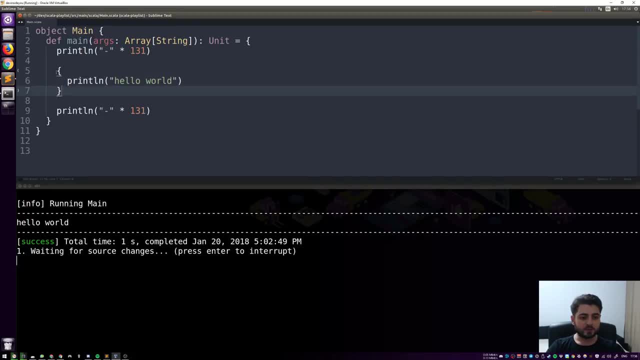 The first thing that we're gonna do today doesn't have anything to do with higher order functions. I'm sort of tired of having this scope here just to have those hyphens. So what we're gonna do over here? so, instead of having all of this, we're just gonna call. 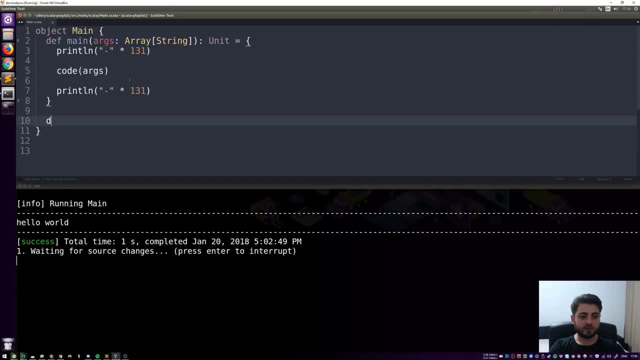 a function called code and we're gonna pass in the arguments And over there we're just gonna define this function, which is gonna look exactly like the main function. Turn to unit oops, unit equals, and it will, in this case, just to print line. hello world. 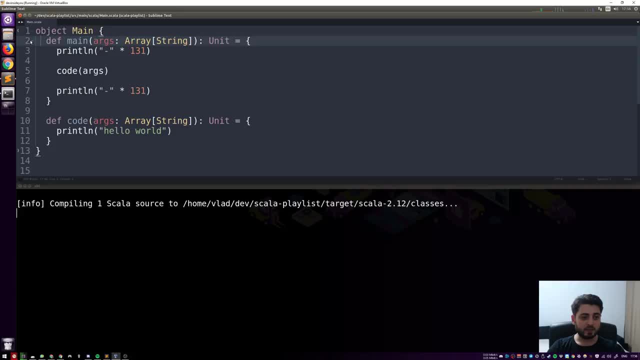 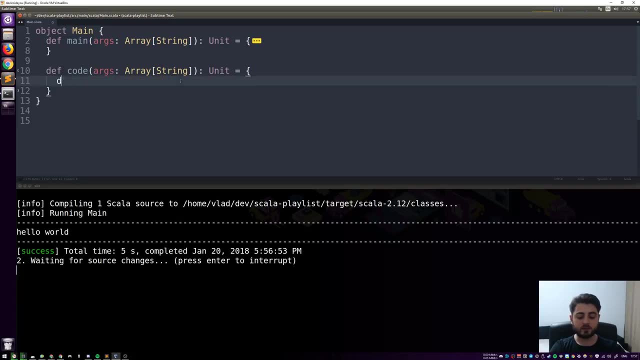 So the result should be the same, but now it allows me to just collapse the main function and all our code is just gonna be over here. Let's start with something simple. Let's define a method called plus five. It will take some input. 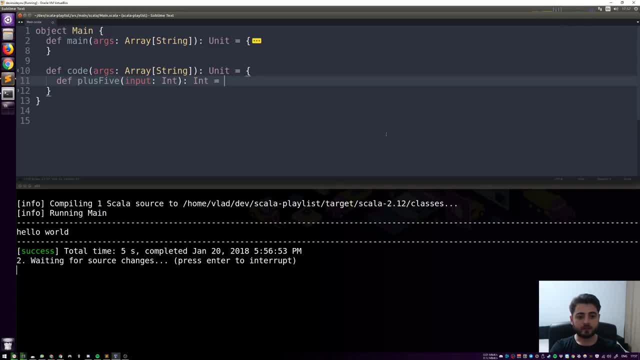 Which is an integer, and it will produce an integer right, And all it will do is it will do input plus five. Not sure why it's so hard to find the plus character. All right, so we have this function, and what I wanna do here is I wanna have a rendered. 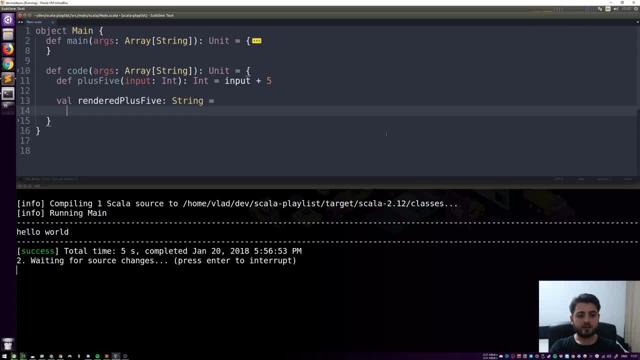 plus five, which is gonna be a string, right? And I just wanna print out whatever's gonna be there, okay? So what I wanna have here is just a string, right? So I'm gonna have a string. I want it to say function, and the name of the function is plus five, right? 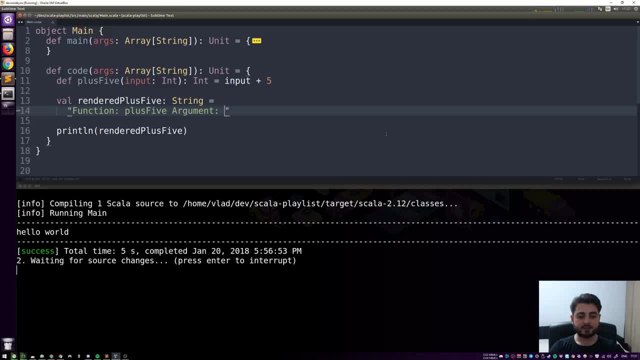 And I wanna say that the argument is, let's say 10, right, And the actual result is: well, 10 plus five is 15.. So this is what I wanna have right. But notice that in this example we're not even calling plus five, right. 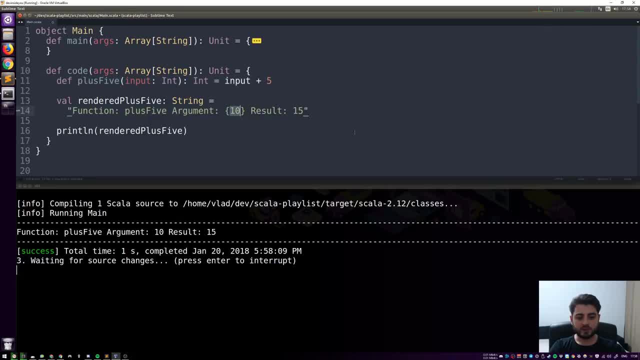 So let's first do this right And actually Get some sort of like a better highlighting. So if you use string interpolation right, then we're gonna see our values right. So we have 10 over there and 15 over there. 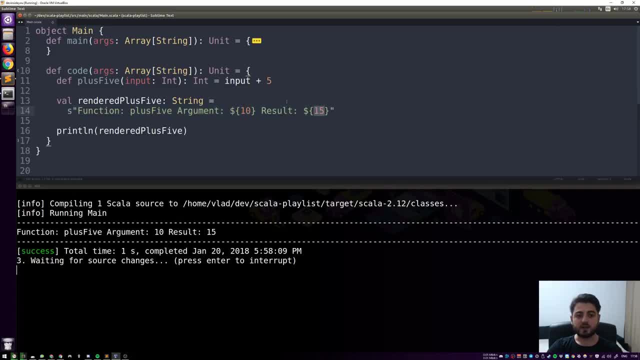 But we produced this 15 ourselves, right? So in our hands we did 10 plus five. What we actually want is we wanna call plus five with a 10,, right? So we're gonna have plus five with a 10, and the result is the same. 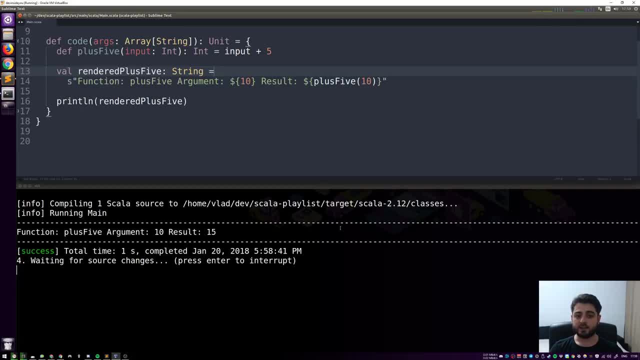 So what I wanna have now is I wanna have another function of exactly the same kind. So I wanna have another function that takes an int and produces an int. This function is just gonna take the input and divide it by two. okay, And I'm just gonna copy-paste everything. 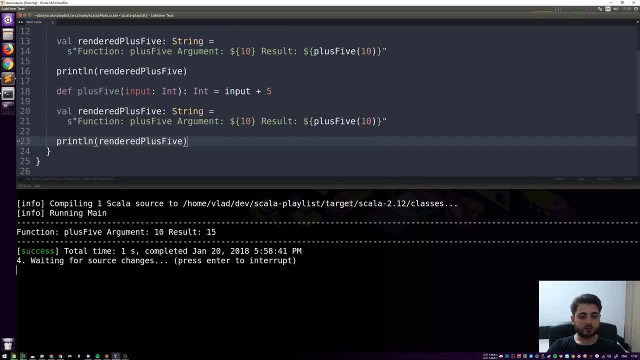 So we're gonna have everything twice right. And everywhere where we say plus five, we're gonna say divided by two. okay, And this is not gonna be a render plus five, this is going to be a render divided by two okay. 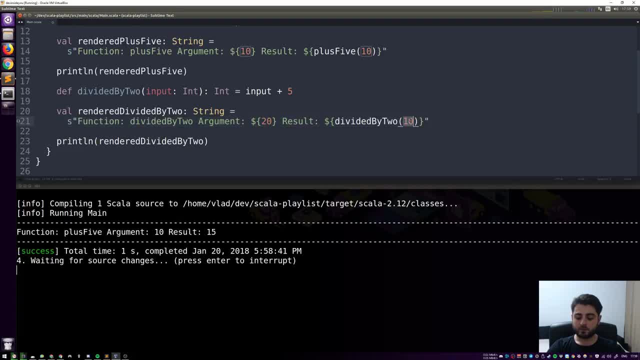 And the argument is gonna be 20, and it will actually divide it by two. okay, So this is what I wanna have. So, for a plus five, we give it a 10,. 10 plus five is 15.. For, divided by two, we give it a 20,. 20 divided by two is 10, okay. 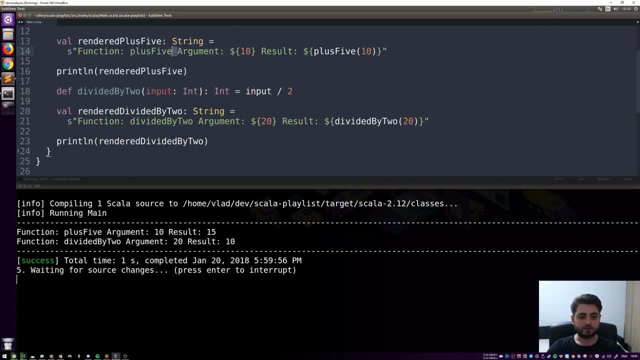 And I sort of wanna make it look like a table, and therefore we're gonna, instead of a space over here, we're gonna- use a tech character and we're gonna do the same thing over here. right, And because of that, we're gonna do the same thing over here. 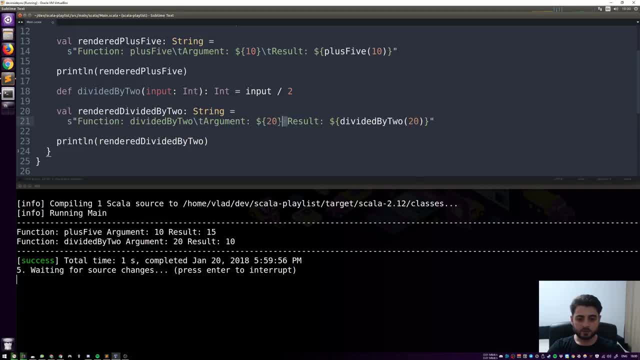 So we're gonna do the same things down there and over there. whoops over there as well, okay? So if we render it now, it's gonna look more like a table. Let me now rearrange the code a little bit. 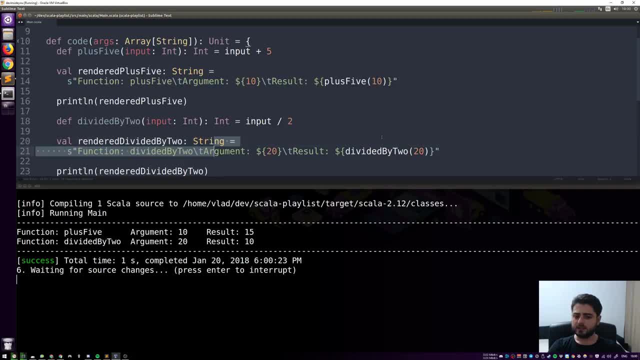 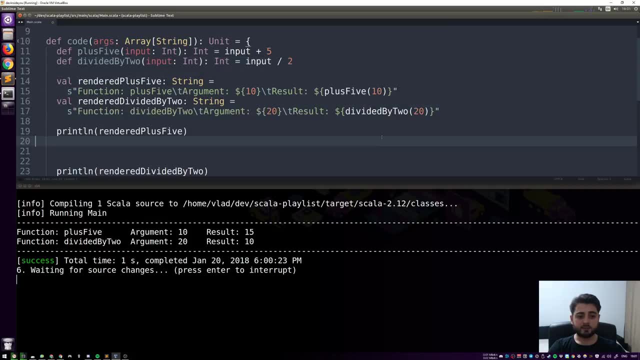 And, by the way, this is already an 11th video, I think, in this video in this playlist. So by now you should know that programmers don't like repetition. okay, So now you can kinda see all code in the same screen and you can see the repetition a little. 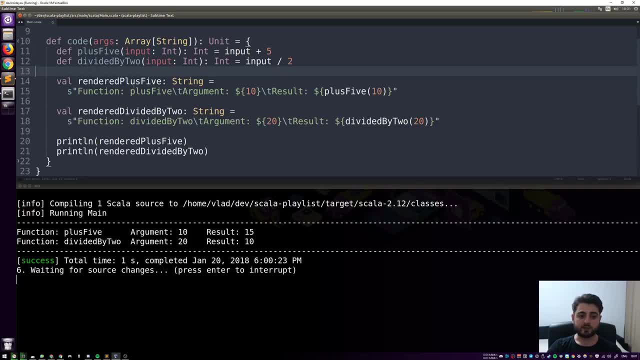 bit better. So what we wanna have now is we wanna have a function rendered that will get a few arguments and it will produce this sort of string for us. okay, So let's define it over here. By the way, so as of right now, I hope I didn't break anything. 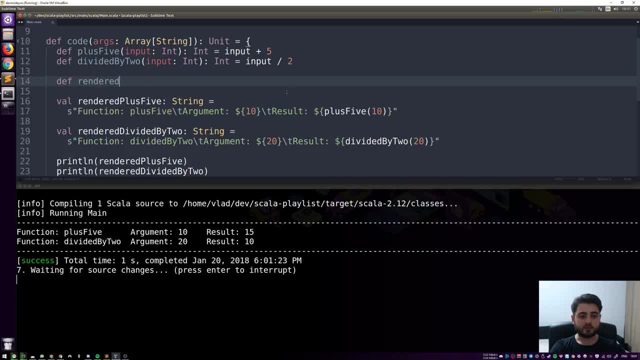 Yes, I did. Okay. so we're gonna have a function called render. It's gonna take a few arguments and then it's gonna produce the string for us, okay. So what it will do is it will actually let me duplicate that. okay, let me put it over. 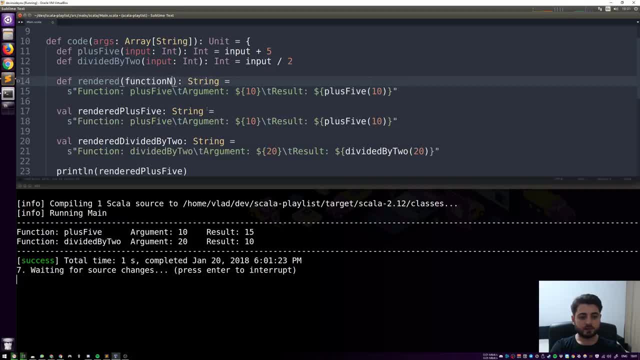 here. So it will take the function name, right, Function name. Okay, So it will take the function name, which is a string, and it will use it over here. right, So this is going to be function name. Then it will take the argument which is a integer- okay, and it will just use it over. 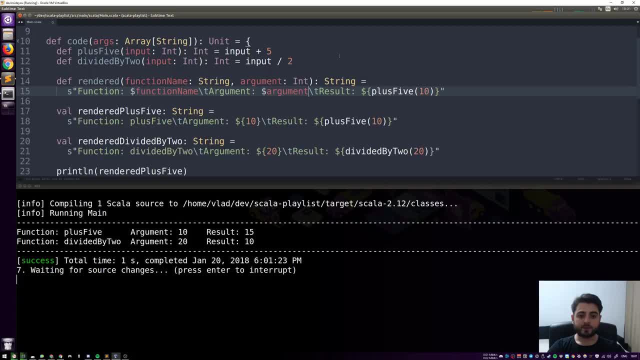 here And because it's one thing, we don't need the curly brace- okay, And it also is going to take the result right and it will use the result over here, okay, So let me see if that compiles. 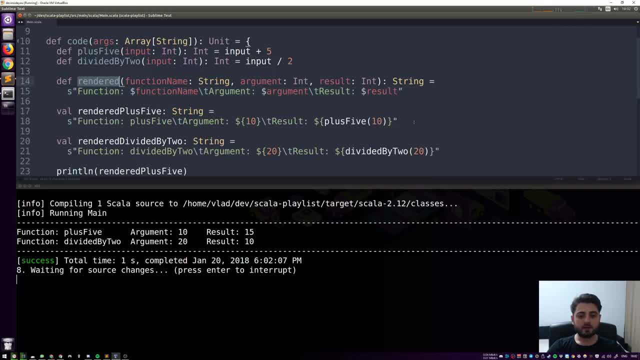 So we're not calling render yet, but at least now it already compiles. So now let's take this one, Right? Let's just copy paste it over here. Let's call this one old, okay. So now this one is called okay. 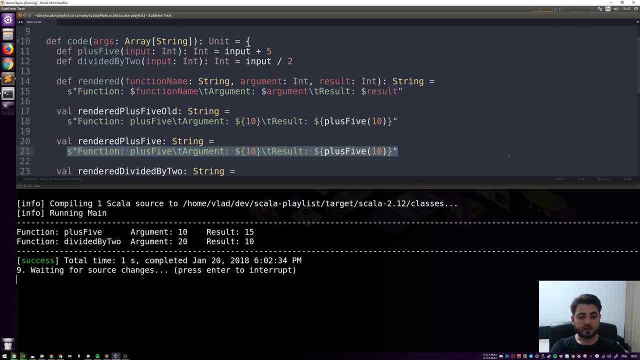 So now we're just going to replace this with the call to rendered. So we're just going to call rendered and the function name is going to be plus 5,, okay, And the argument is going to be 10, and the result is going to be plus 5 with a 10.. 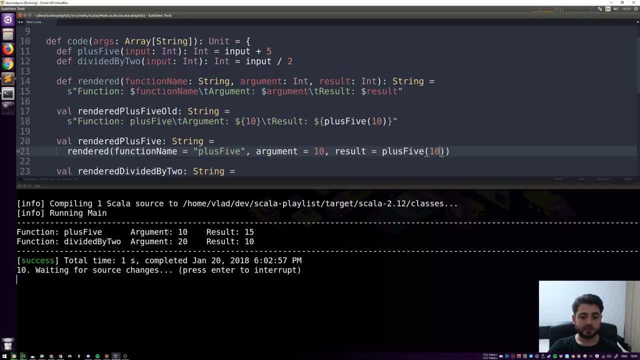 And now, because what we're seeing over here is that the argument is going to be 10, and the result is going to be plus 5 with a 10.. And now, because what we're seeing over here is the same, we know that we did it right. 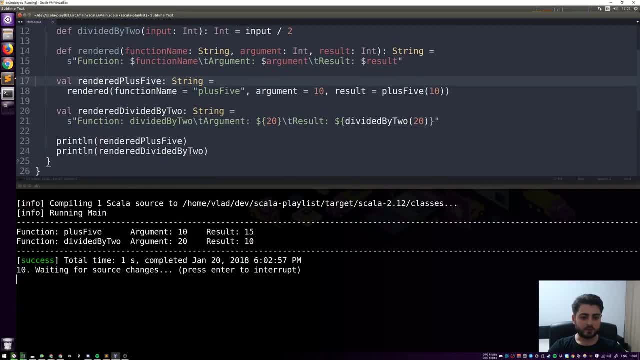 so we can remove the old one, okay, And we can also remove the. we can also replace this one, okay. So let me just duplicate that. So this is now divided by 2, and a 10 becomes a 20, and this also becomes divided by 2,. 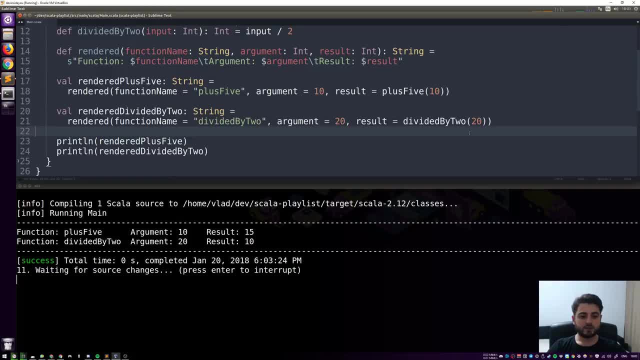 okay, So we can remove the manual string. Let's also real quick remove the named parameters. So let me see, Maybe I can do this, Okay, And that, all right, And the same thing over here, this and that, And now we can have them in one line like this, and let me indent it a bit like that: 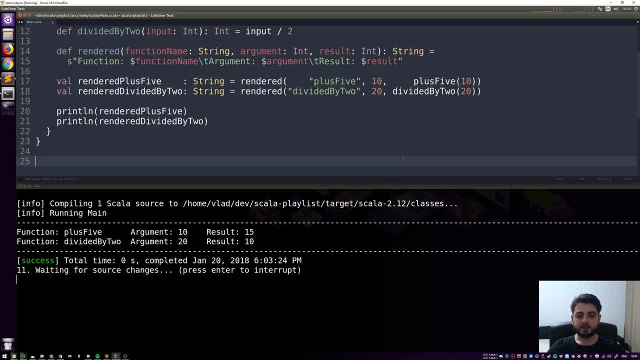 so that we see it better. okay, So this is what we have now. Now, the thing is that, first of all, this is already really good, but we still have duplication, right. So, first of all this thing: it's sort of lonely. 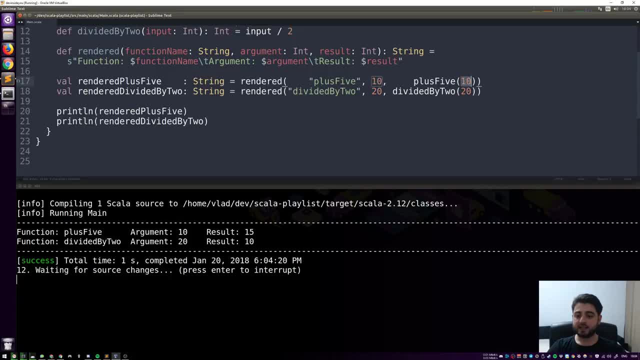 It's sort of looks like duplication, but it's actually not, whereas this one actually is duplication. So this is not duplicated, because actually we're going to call this function, for example, plus 5, right, And this one is divided by 2, okay. 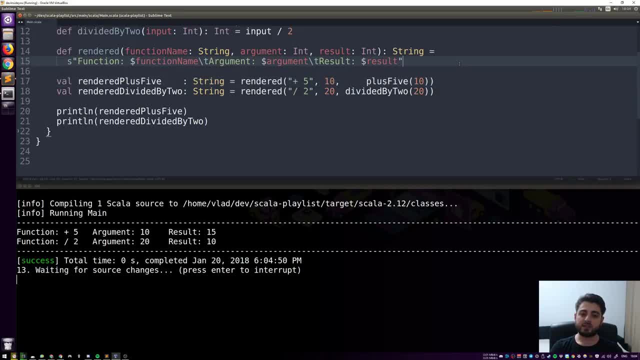 So now we can do this right. So now it should be more clear that this is actually not duplicated. This is more like a coincidence, okay, But this 10 is actually duplicated, and this is where we're going to start using higher. 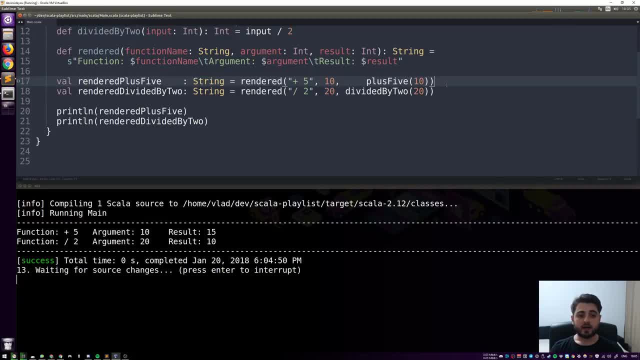 order functions and see their value. So in this example, we're going to use higher order functions. Okay, To get rid of some duplication, right? So our code is going to be more concise. but do not fool yourself, This is not the only benefit of higher order functions. 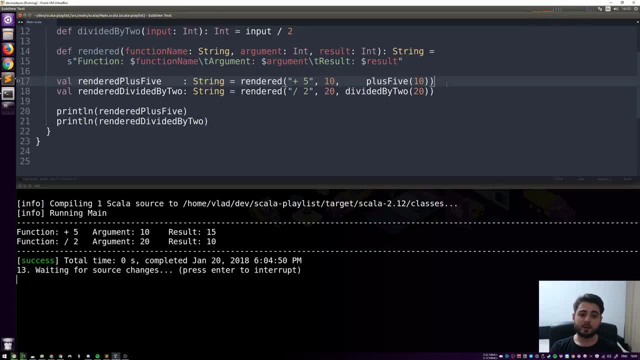 The list of benefits just goes on and on. It's just that I picked this example because I think it's a really good one for education purposes. okay, So in this case, higher order functions are going to help us to get rid of duplication. 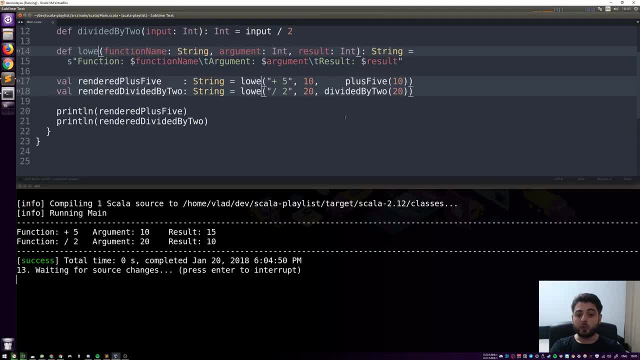 So our rendered function is actually a lower order rendered right. So there's, I'm not really sure if there is such a thing, It's a lower order function, right. But I thought if there is this thing like a higher order function, probably the function. 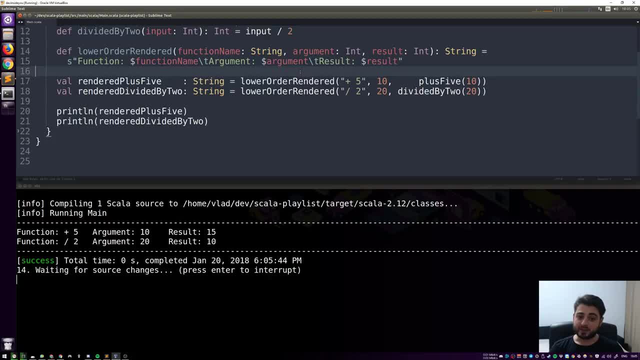 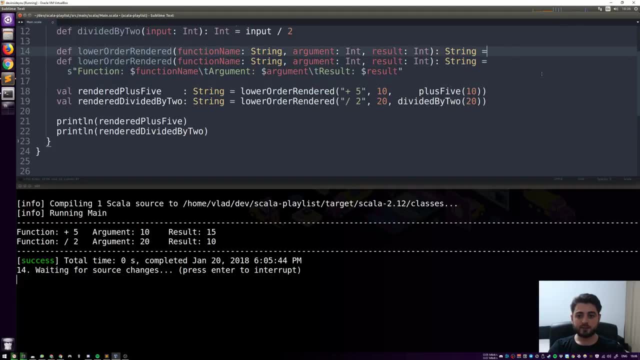 that does not take any functions as arguments should be called lower order rendered, right? So okay, So this one is called lower order rendered, So let's create a higher order rendered. So I'm just going to duplicate the signature, right, And I'm just going to call it higher order rendered. higher order rendered. 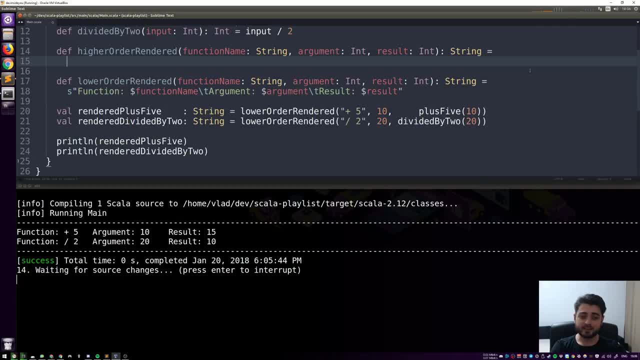 So I'm not going to make a higher order function out of it yet. I just want to keep it compiled right, So I'm just going to call lower order rendered. Okay. So I'm going to create a higher order function with function name, argument and the result. 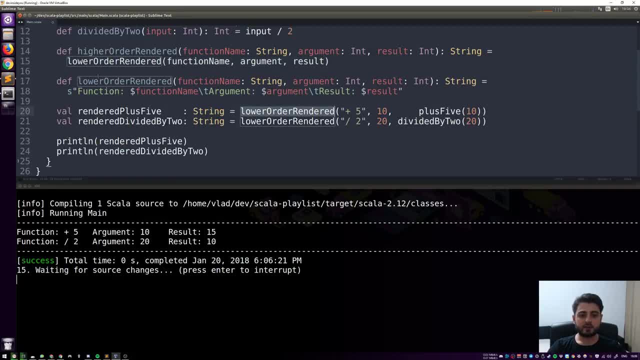 So, as of right now, over here we're calling lower order rendered, but now I want to call higher order rendered. right, And the result should be the same, because this function as of right now. it just delegates to this one, okay. 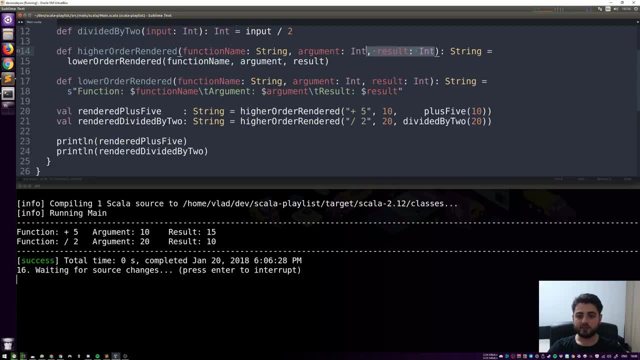 But this is not what we want. So what we want is: let me remove the last parameter. What we want is let me use a name parameter over here. So what we want is we want to have something different here and something different over. 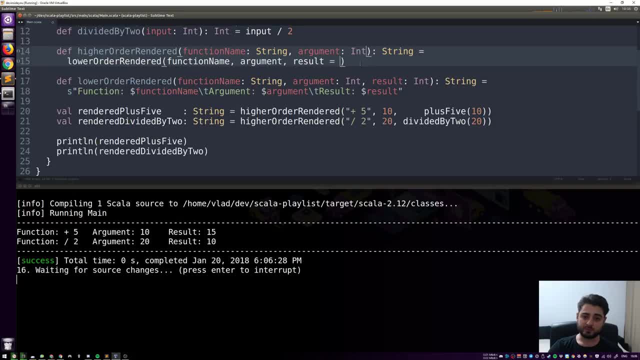 here Higher order functions. So let's say that this is an argument. Let's say that this is an argument, Okay. So let's give it one. So let's say that this third argument is actually a function, In this case, a function that takes an integer and produces an integer. 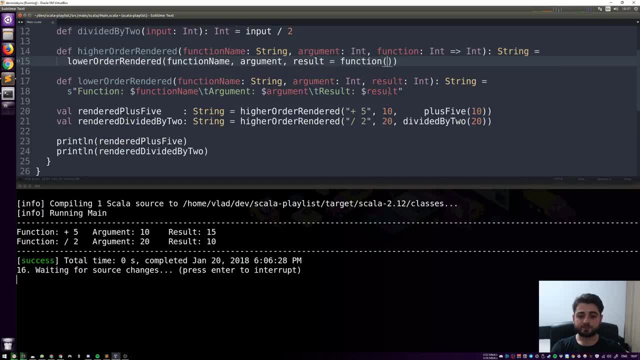 Okay, And the result is just going to be this function, which gets this argument passed in. So we're just applying this argument to this function And because of that, when we call higher order rendered, the last argument is now not an integer. 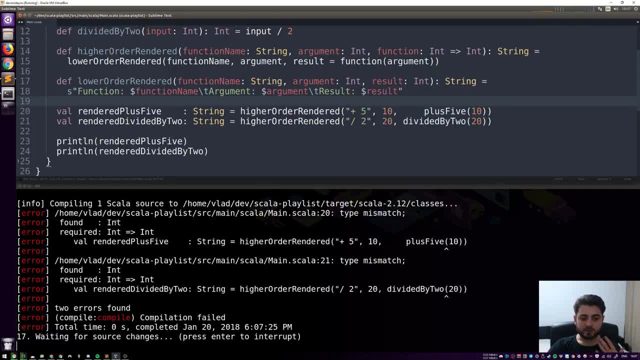 Right. So if we compile it now, it's going to tell us: hey, we found this function, Okay, We found an integer, but we actually want a function that takes an integer and produces an integer. Well, plus five and divided by two, are those functions? 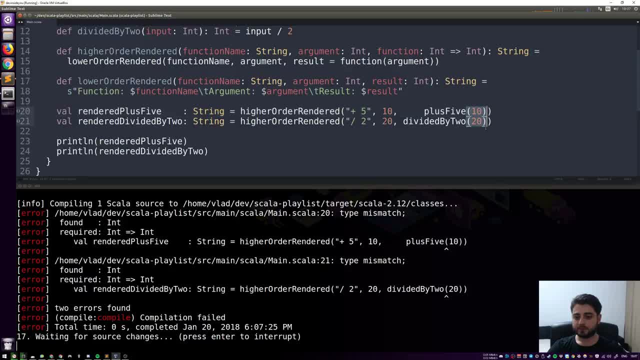 Right. So all we need to do is we need to remove the parameters Right, We need to remove the argument, And this is what we wanted to do Right From the beginning. we wanted to get rid of this duplication Right. 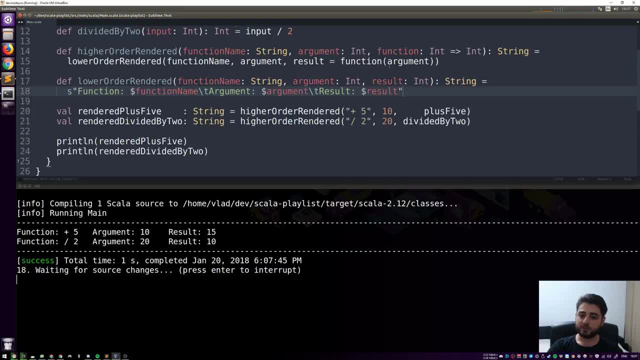 So now higher order rendered will call this function for us, Right? So it will call plus five, and then it will call divided by two, and it will produce exactly the same result. Before we continue, Let's clean this up a lot. So, because it gets smaller and smaller and smaller, let's just not have those extra vowels. 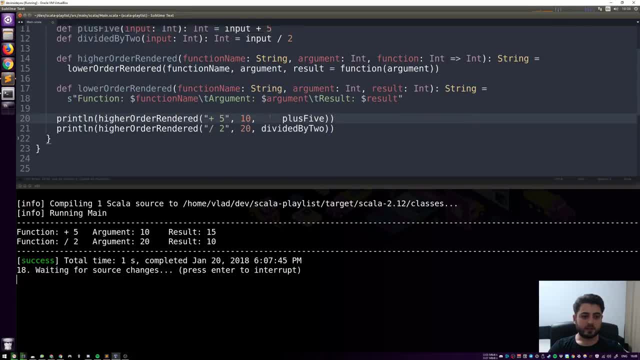 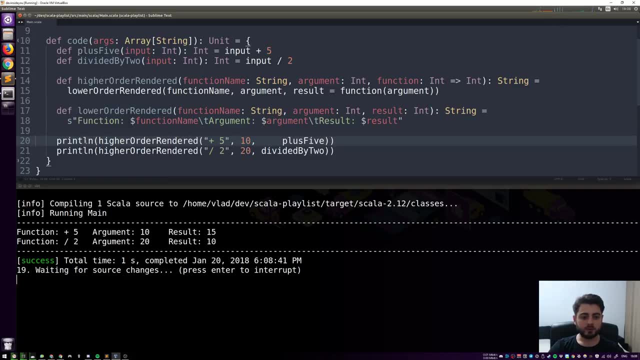 Let me just inline those two so that we can remove them and then we can actually see most of the code on one screen. And also, let's define a function show- which will do print line and higher order rendered at the same time. So we're just going to duplicate this one. 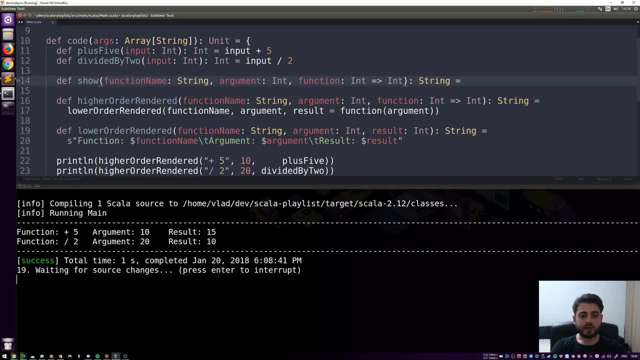 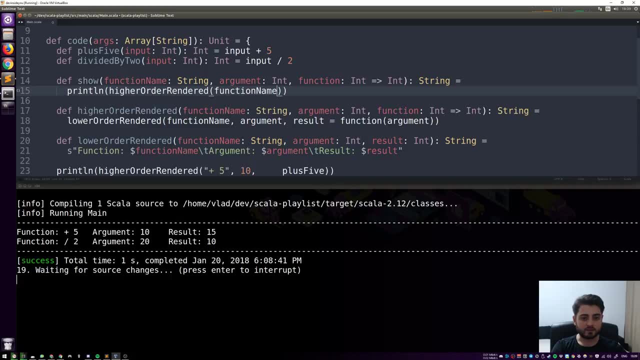 Right, And we're just going to call it show Right, And all it will do is it will do print line Right. So we'll just call higher order rendered for us and we'll just pass everything. sorry, function name argument function to it. 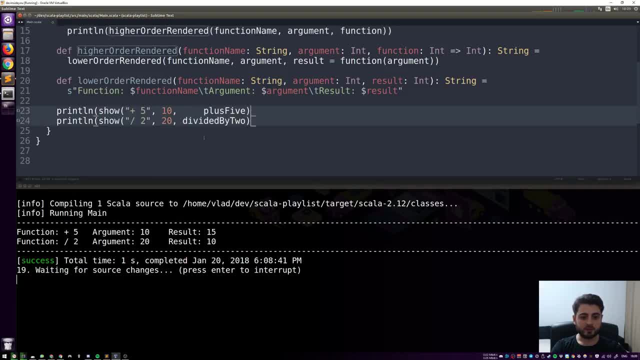 Okay, So we're just going to use show over here and now we don't need the closing brace and now we don't need the print line. Okay, So the show is doing the print line for us. Okay, It's exactly the same code. 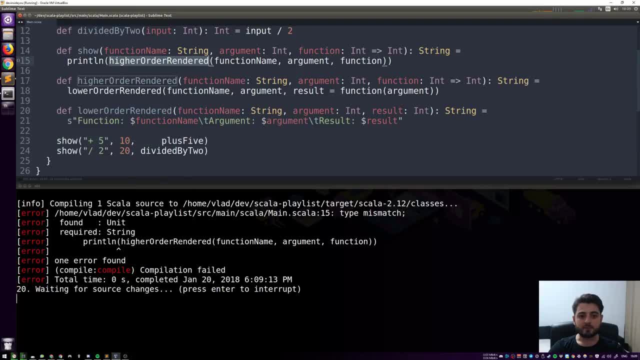 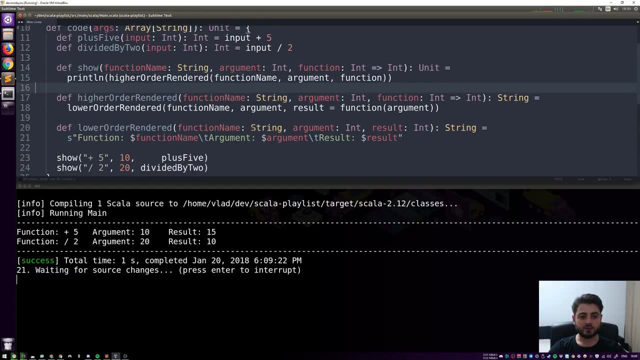 And what did I do wrong? Oh yeah, because it duplicated it. it has to return a unit. Okay, Because it's just doing a print line, Okay. So this is exactly the same code, just rearranged a little bit. Also, since we're in Scala and Scala has function literals, look at these two functions: they're. 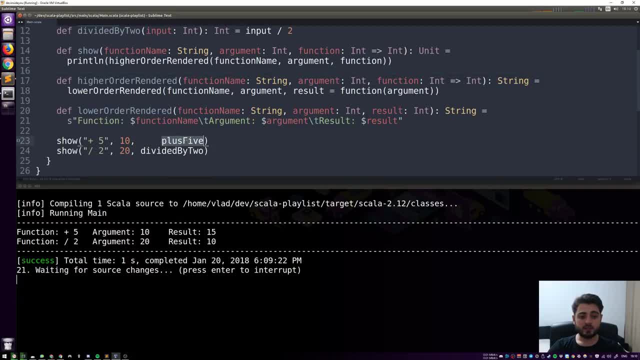 actually really tiny, We don't need extra definitions for them. So we can just do this: Whatever comes in two plus five And over here, whatever comes in two divided by two. Okay, And let's do this now, And it should be exactly the same. 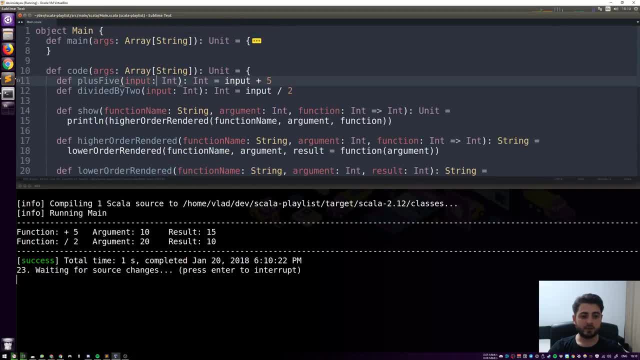 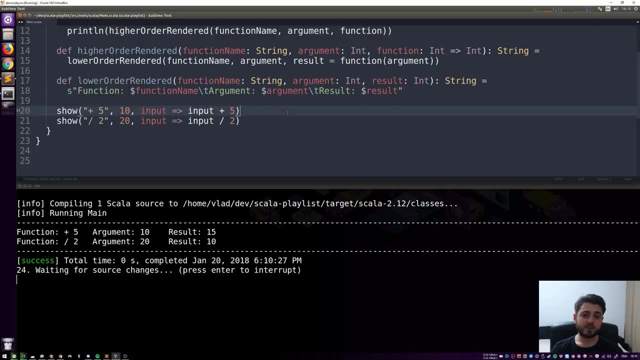 Oops, there's a space over there. Yeah, so it should be exactly the same. and now we don't even need these, Right? I already said this in the very beginning, but really know the difference between functional literals and functions as object, because most languages actually have functions as object. 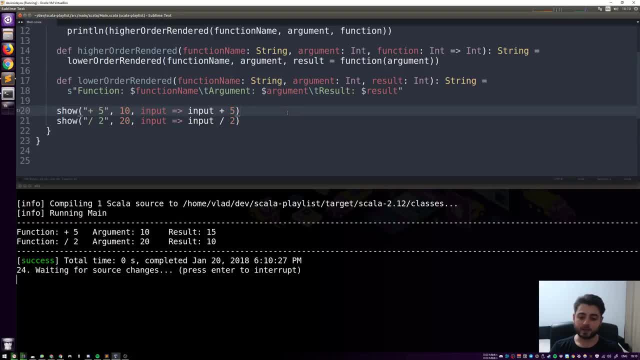 in one way or the other. Maybe they're sometimes hidden behind stronger syntax constructs, but not all languages have functional literals. So only because your language doesn't have functional literals does not mean that it cannot have higher order functions in one way or the other. 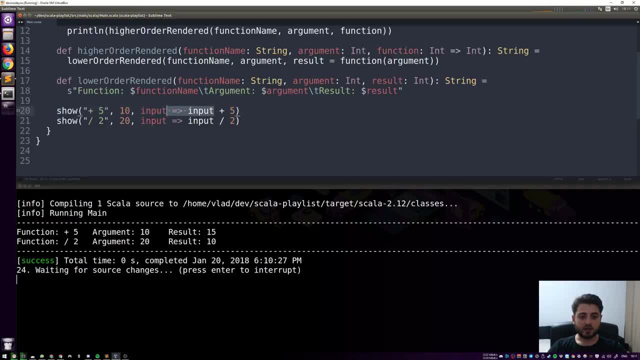 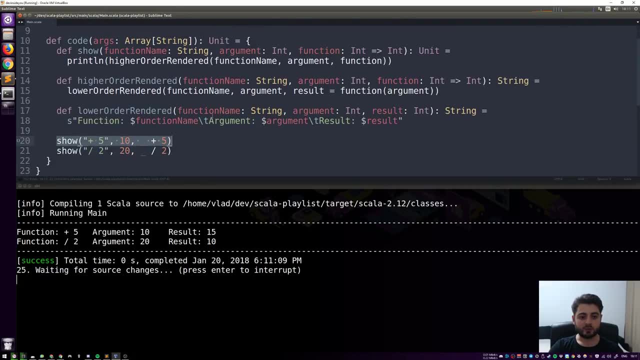 And, by the way, remember, Scala has this awesome syntax where we can just say whatever comes in: Do plus five or do divided by two, Right? So look at this line. It's just so tiny now, And our code is just a few lines long and it's doing virtually the same thing as it. 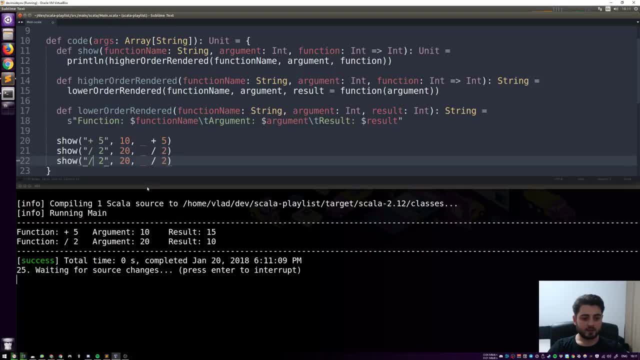 was doing before. Let's have a few more examples. Let's have a- I don't know, let's have times three, for example, And let's give it a two as an argument. So let's also do a mod. Let's do mod two. 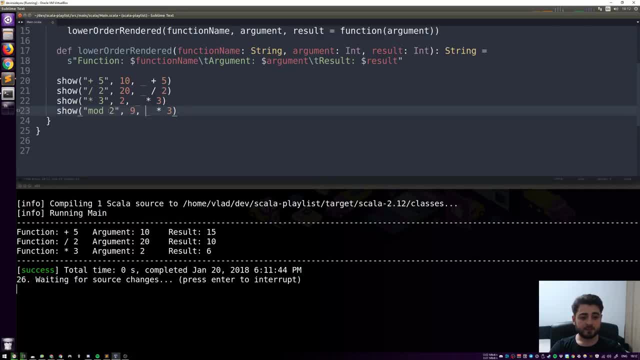 Right. The argument is going to be: I don't know. let's say nine And it's going to do mod two. Okay, And so, yes, nine, mod two is one. Let's do the same one with a 10, actually, right. 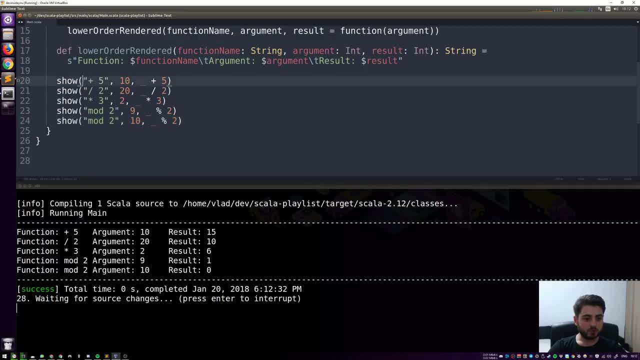 And now, because we have some duplication, actually hold up, let me do, let me do that and that and that, All right, So now it sort of looks like a table. So now we have a little bit of duplication over here. 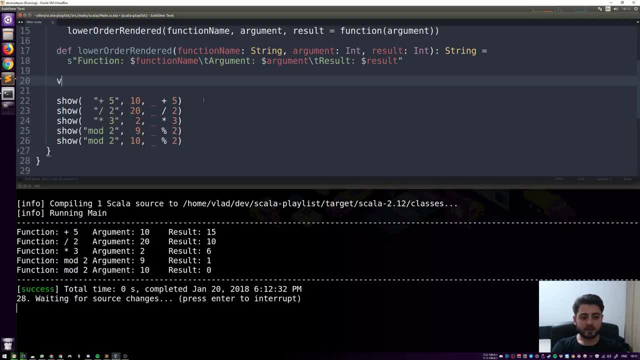 Right, And now you have a choice, right. So you can. You can either have a function mod here, right? You can have it as a function that takes an int and produces an int- right, And then you can just take this and paste it over here. 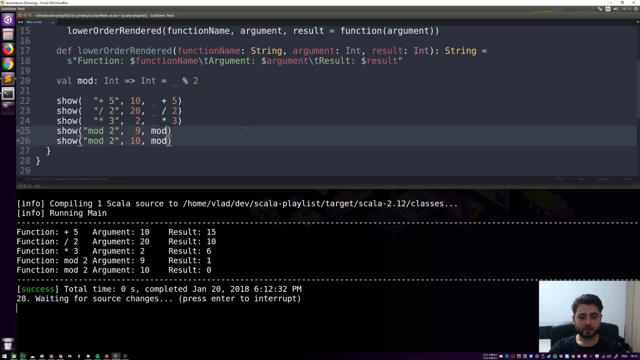 And now over here you can. you can just use mod, right. So you can either do this or you can use the other syntax right. Let's comment this out. You can use the method syntax right. So you say: whatever comes in, right and integer comes out. we're just going to do. 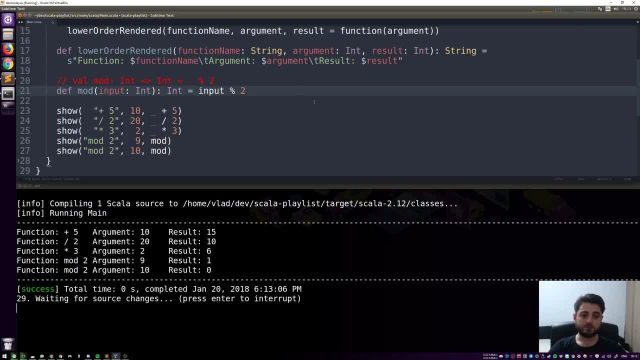 input. Input Modula, Modula two: Okay, And notice that, even even if we do, even if you use one character- and I'm not sure if this is a coincidence or not, So let's, let's just use an X over here instead of, instead of input. 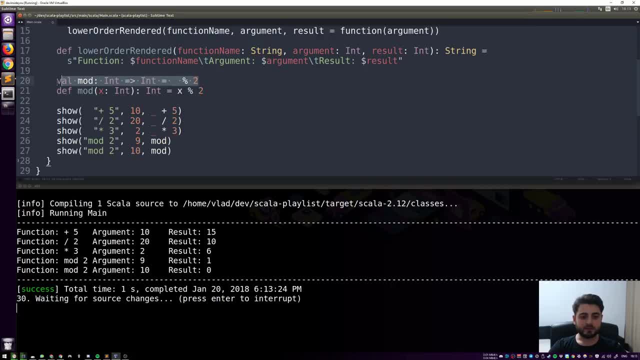 Let me uncomment that. Look, this one is still shorter, right, It's kind of funny. Also, let me. let me do this that you may be- you know, you might not be used to to those kinds of things- Let me do that. 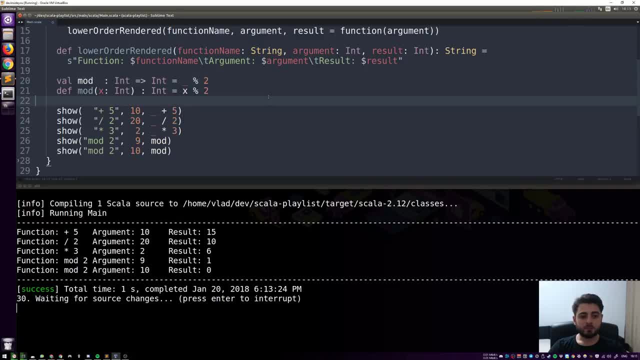 Over that, So that it sort of looks Okay, It looks kind of similar, but we can't have both of them, right. We have to decide. So are we doing this one and let the add expansion to convert it into a function, or let's just 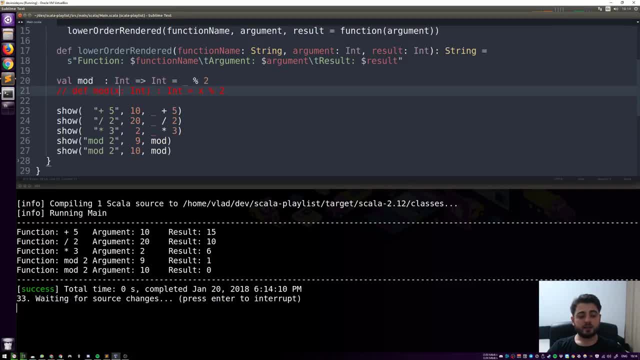 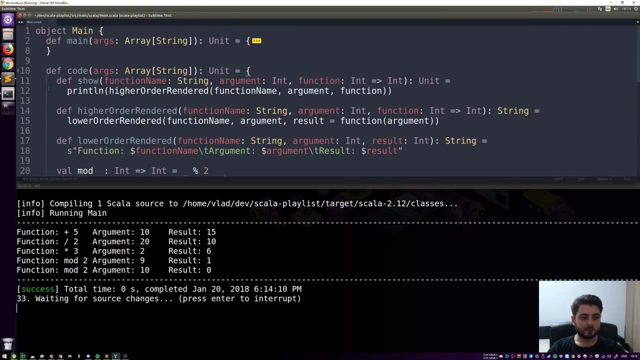 give it a function directly and have that. Okay. Remember, in the video about recursion we defined functions- factorial and Fibonacci- and they just happen to have the same structure, right, And some integer comes in and some integer comes out. So let me just copy paste them from this video and I'm just going to insert them somewhere. 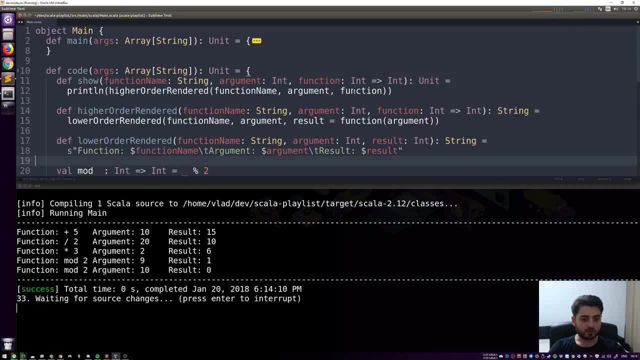 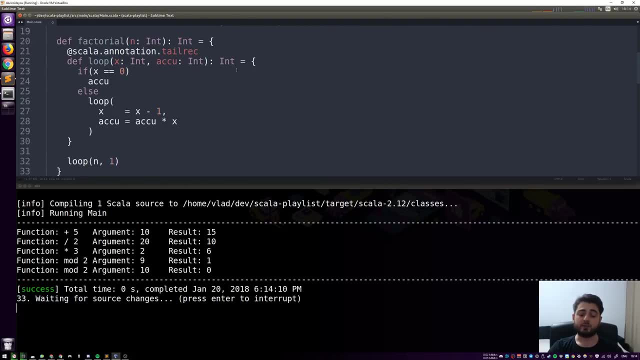 somewhere at the top, somewhere, I don't know, Over here. Let's have them over here, right? So you don't need to understand the implementation, you know, just rewatch that, that other video. In fact, I'm just going to collapse them. 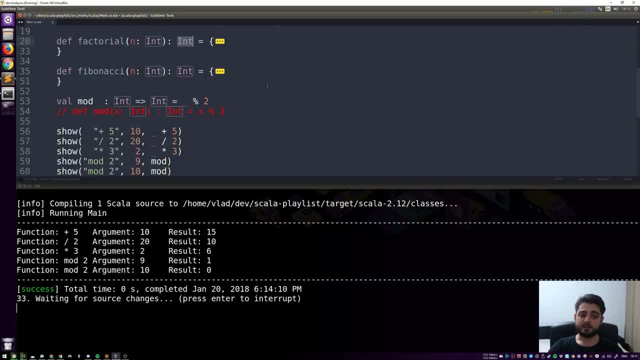 The only, the only thing that is important to us is that the integer comes in and then the integer comes out, right. So what we can do now- assuming that it compiles- and yes, it compiles- what we can do now is: 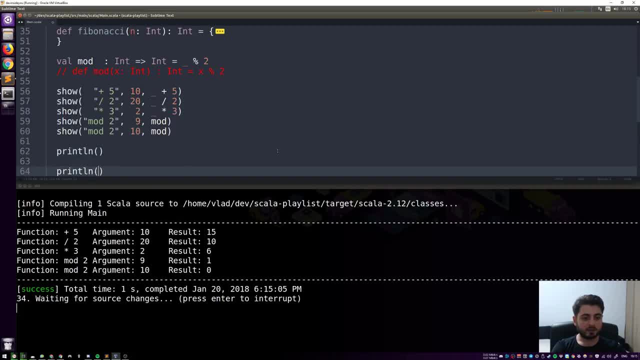 let's have an empty line over here, let's have a print line, Okay. So the first one is going to be a factorial Okay, And the argument is going to be zero and it just should just call a factorial Okay. And let's do it a few times with a one and with a two, and we should see all right, obviously. 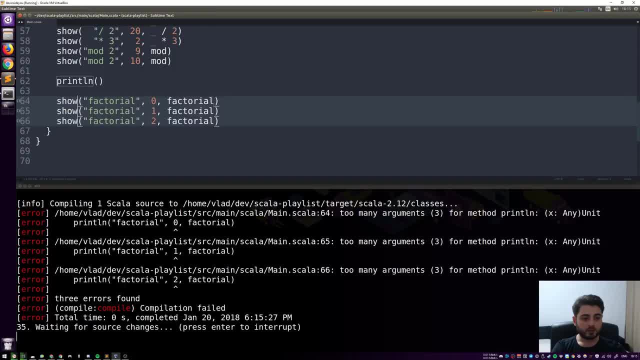 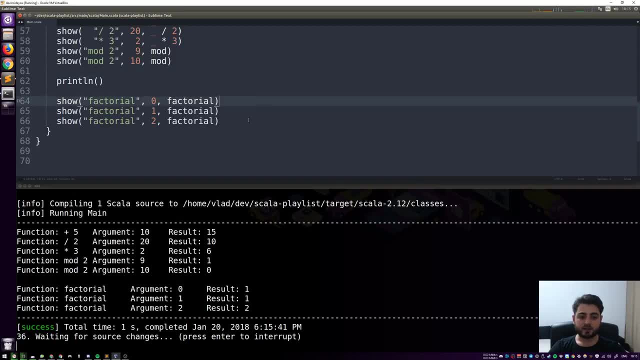 I didn't want to call print line, I want to call show. whoops, sorry show. There we go. Okay, So a factorial of zero is one, factorial of one is one, factorial of two is two. That's not very spectacular. 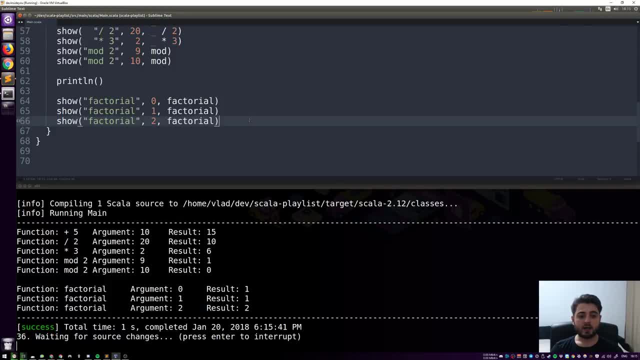 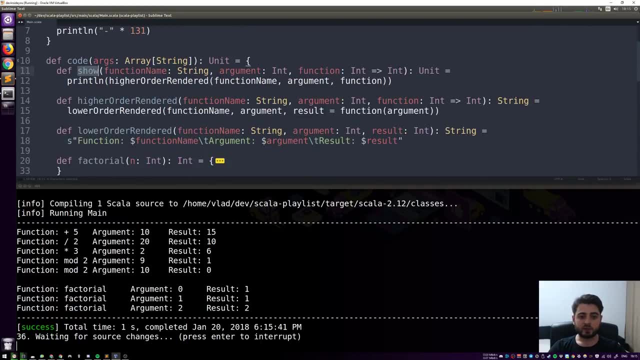 So in fact, we want, we want more numbers. So what we should do now is we should define another function That can not take only one argument, but multiple arguments right. So over here, show: takes a function, function name. 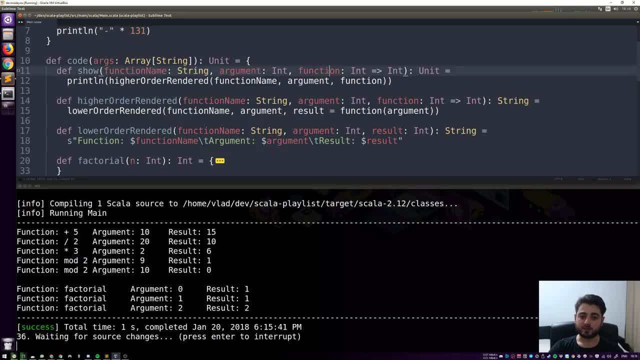 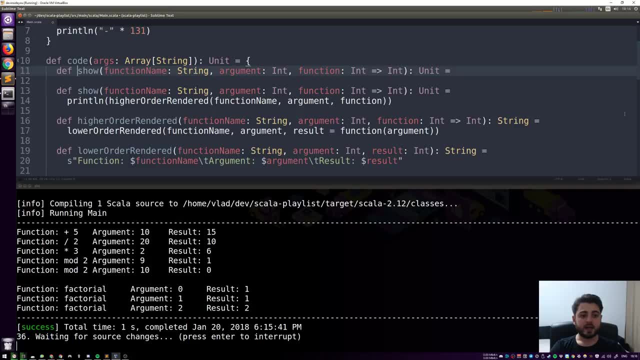 It takes one argument and then applies this one argument to this function, right, Just just once. Okay. So what we should do is we should define our own function, yet another one, and we should call it show range, right, So we'll take the function name, but then we'll take a bunch of arguments, right? 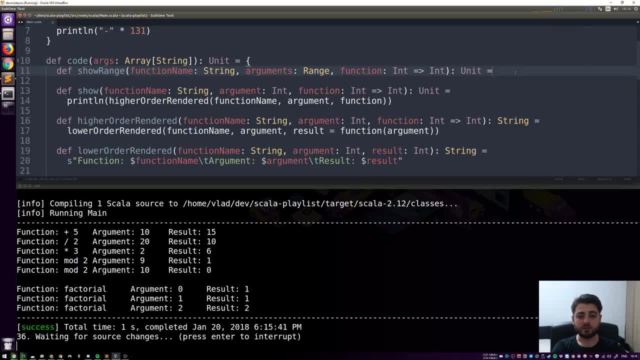 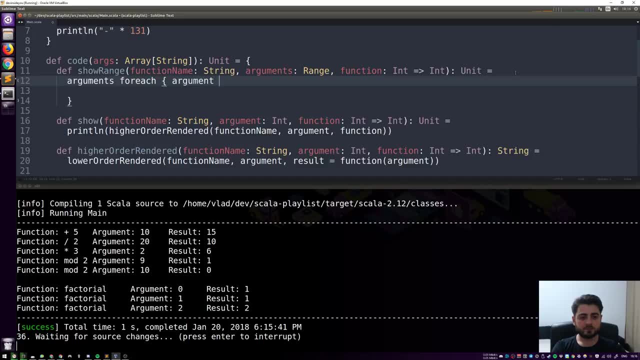 A whole range of arguments, Okay, And the function, and then it will just go through this range. right, We'll just say arguments for each, Okay, And over here we have the argument and we're just going to show function name argument. 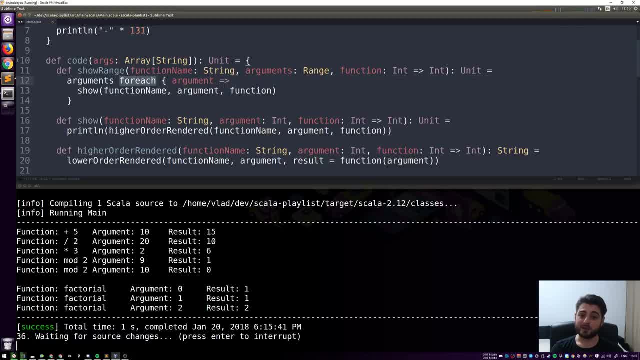 and function- And, by the way, notice, for each itself is also a higher order function, right, So it takes another function as its argument. Okay, So this should compile now. Yeah, So this compiles. So let's go here now. 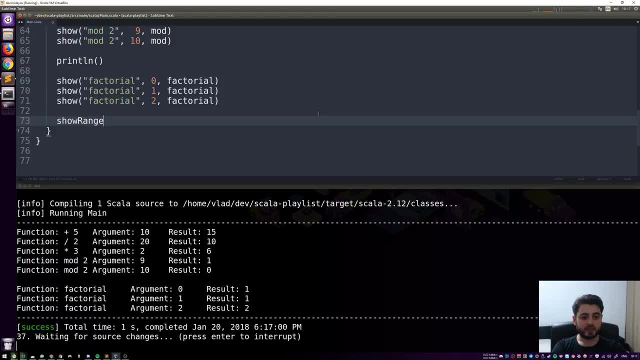 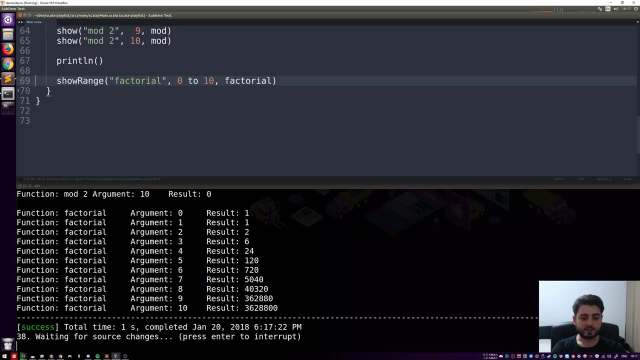 Right. So instead of doing this nonsense, let's say: show range Right And let's say factorial, and the range is going to be 0 to 10, right, Factorial? And let's remove this. Okay, And if I did everything right, then we see factorial from 0 to 10.. 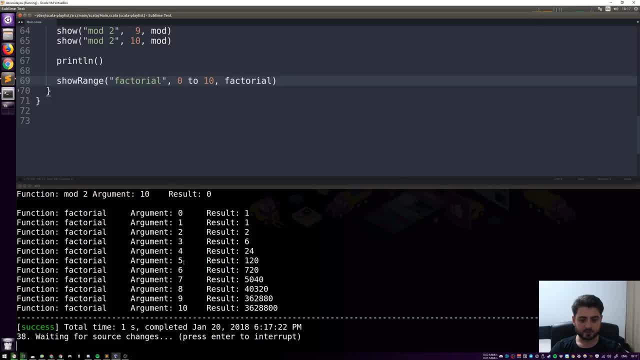 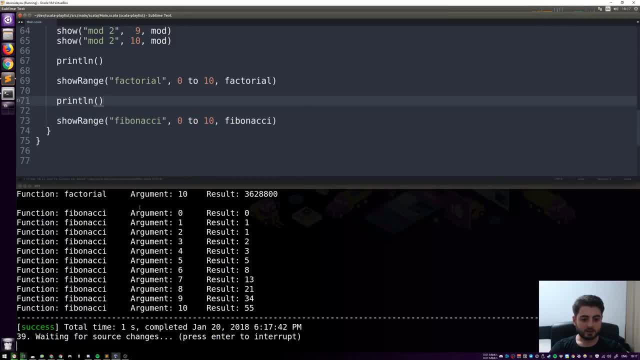 Show range: Fibonacci, There we go 0 to 10.. Fibonacci, I remember, the 7th one is a 13,, the 8th one is 21,, and so on. Yeah, It's all good. Now, these examples might not have been the best ones to show you the value that the higher. 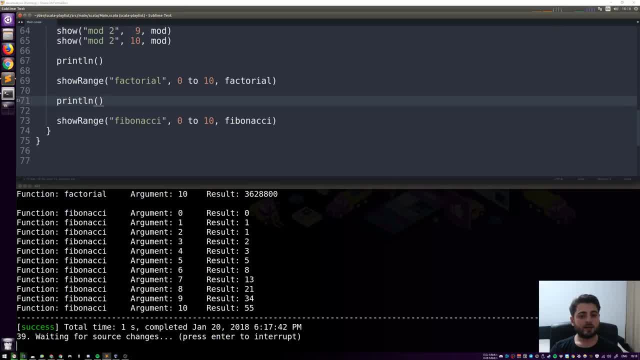 order functions provide, but I believe it was a good way to show you how to drive your design towards higher order functions and also to see how they actually work. As I already mentioned, higher order functions play a very important role in your design. 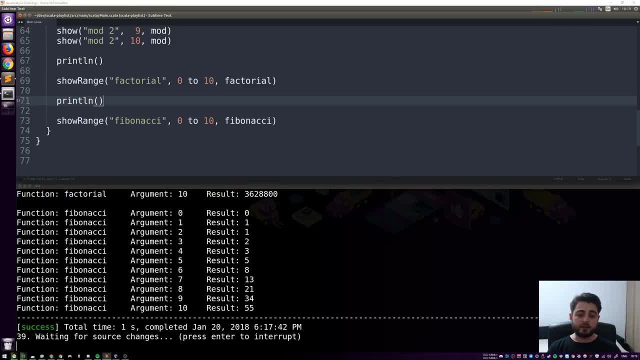 Okay. They're present in virtually every programming language. even though most languages don't have functional literals, It is very common for higher order functions to be wrapped around in some very advanced syntax constructs- right Syntactical constructs that we're going to discuss in the future. 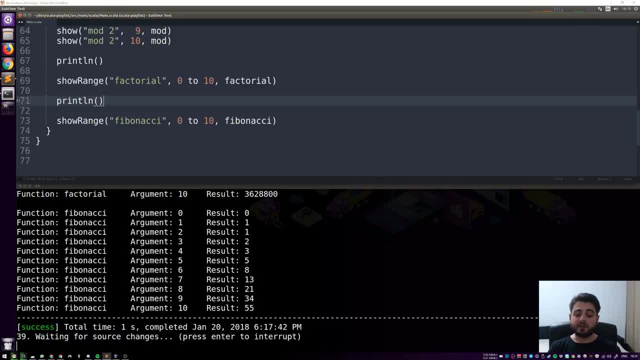 Maybe if you're familiar with object-oriented programming, for example, they're usually hidden behind interfaces and classes, right? So you don't really see them. But in Scala they are so-called functional literals. In Scala they are so-called first-class citizens. 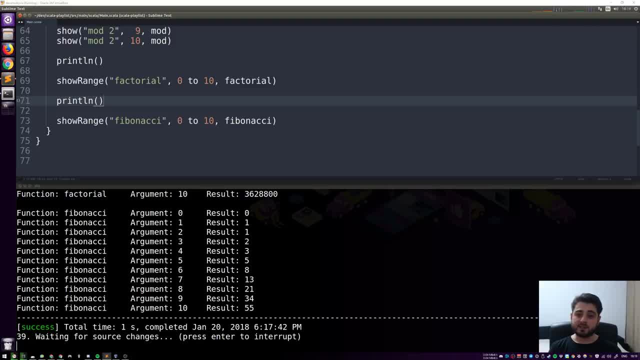 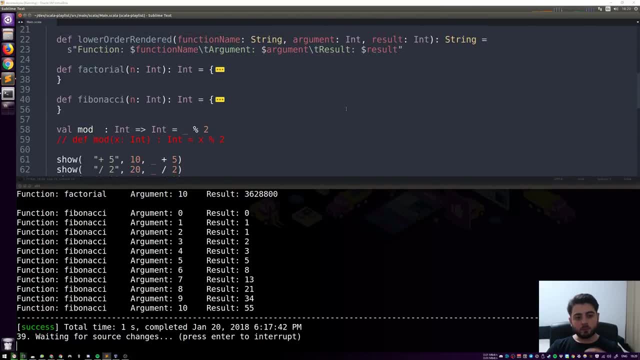 And the first-class citizen is a term that basically means that you can use them as any other data, You can pass them around, You can bind them to variables and so on. Just to show you a little bit more what it actually means to use higher order functions: 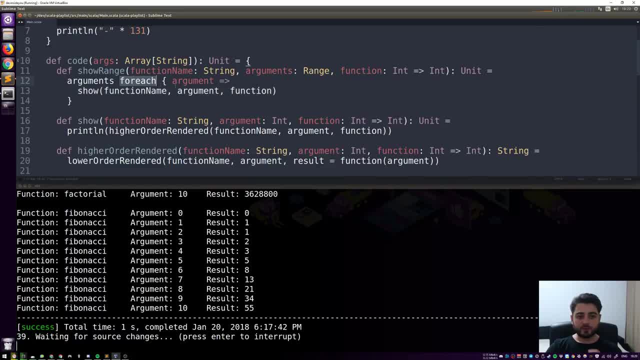 Usually you would have some sort of algorithm, right? For example, for each right, It knows how to go through this range of arguments. right, But it's not an entire algorithm, right? It's a partial algorithm. A part of it is missing. 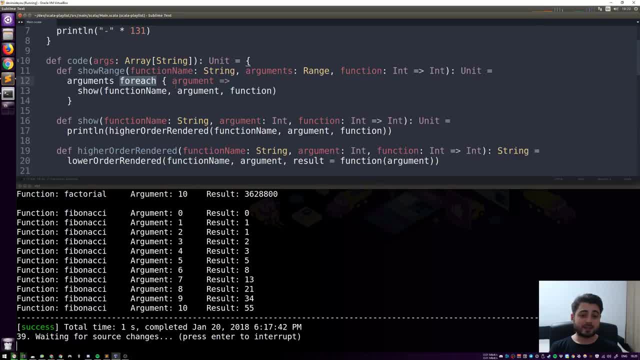 And this part just doesn't exist. It just happens to be another algorithm, right? Sometimes it's tiny, Sometimes it's huge, right? For example, Fibonacci is a relatively big algorithm, In case you're someone who is familiar with object-oriented programming and all the patterns. 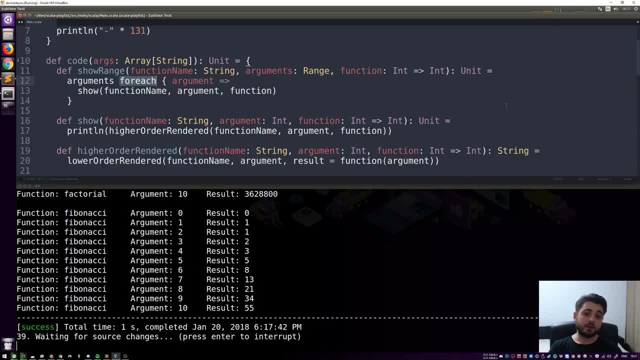 that come with it then in Scala and all other languages that have functions as first-class citizens, and maybe even functional literals on top of them, then they allow you to implement those object-oriented patterns in a way which basically reduces your code to the bare minimum. 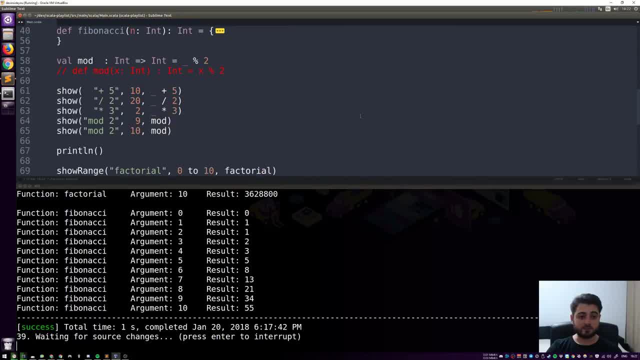 So you can implement these patterns with minimal verbosity, like, for example, over here. right, This is very, very minimal. okay, Now we're actually by the end of this video and finally, I made a relatively short video. Before I leave, I'm going to show you some very special Scala syntax. 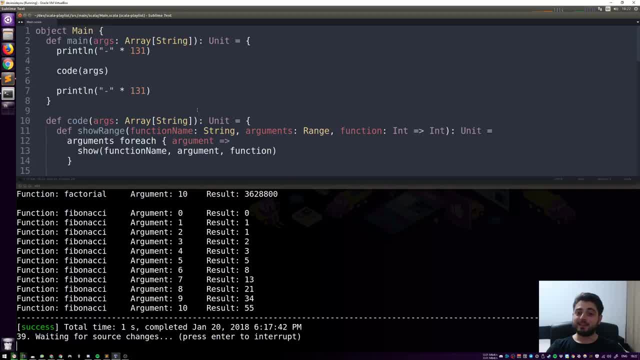 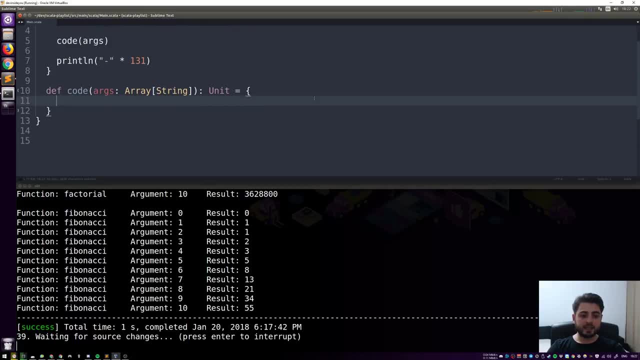 I should have mentioned in my very, very first video that Scala is a very sweet language. It has a lot of syntax sugar, all right. So let me remove everything that we did today, okay, And let me define a function called loop. 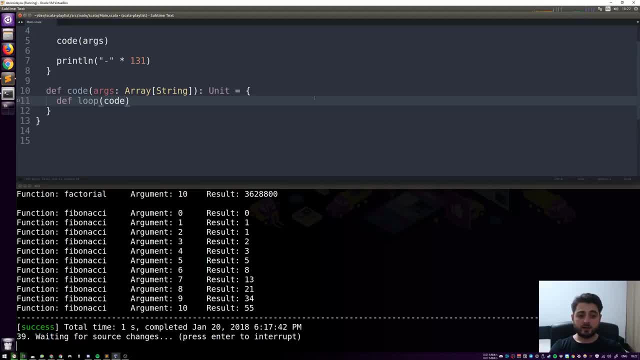 So what loop will do is It will receive a code argument, right? So loop is going to be a high-order function and it will receive a code function which doesn't take anything right and produces a unit. okay, And loop itself will produce a unit okay. 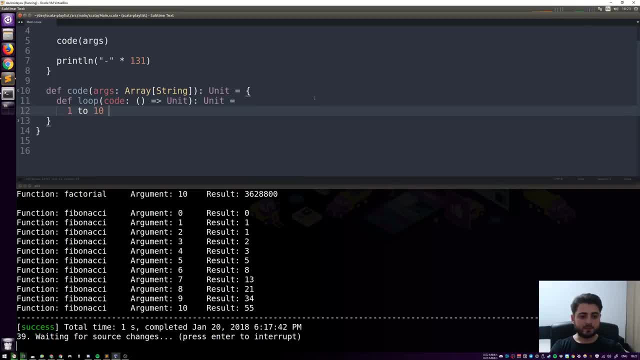 And all it will do is it will just go from 1 to 10, okay, which is a range, And for each iteration, which we don't really care about, right, it's just going to call our code function, okay. 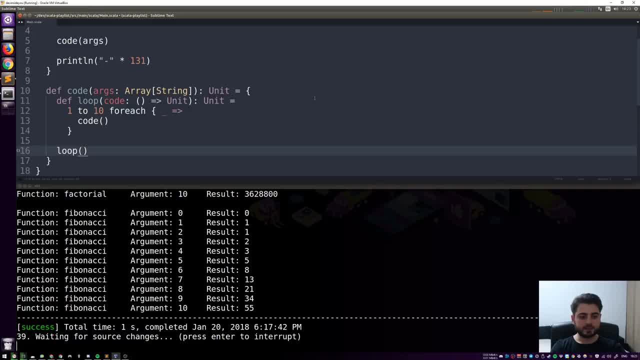 So if you call loop, for example, Let's say loop was a function that doesn't take anything and just prints out. my God, what did I just do there? Prints out high, right, It will print out high 10 times, okay. 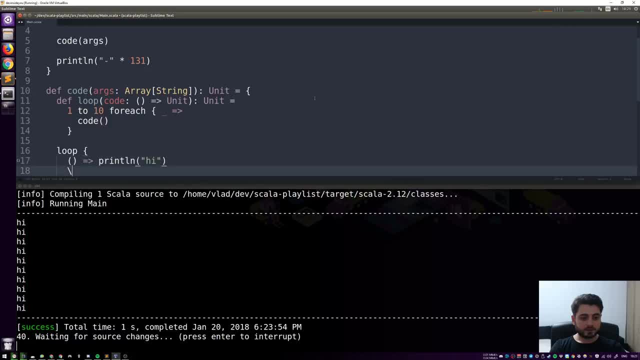 And let's use this syntax over here, right? So remember, if a function receives only one argument, then you can use the round parentheses with curly braces, okay, So let's just have this, And usually when you do this, then you have this part. 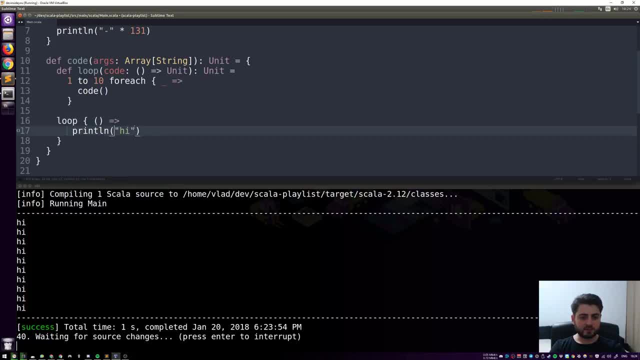 It's very common to have it like this: So let's just have this. And usually when you do this, then you have the, You have this part, So let's just have it like this. right, And you see an example over here, right? 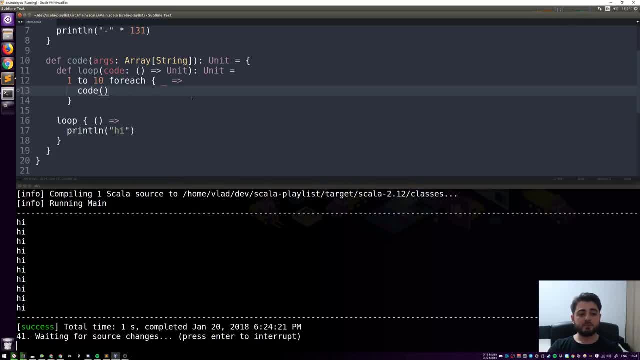 It's very similar, okay, So let's call it like this. So there's a very beautiful syntax sugar for that, okay, So let me call this loop old right, And let me duplicate both of these, both the function and the call of it, right. 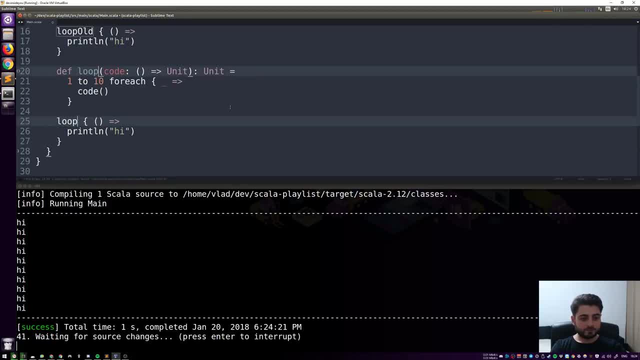 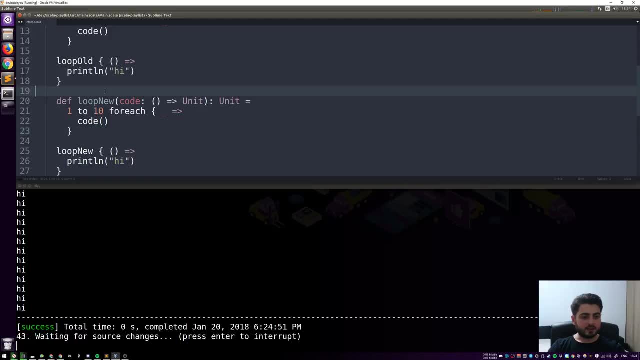 So let's call this one loop new, Come on new, There we go, Okay. So, as of right now, they're still looping. Okay, They look the same, right, And let me actually have a print line in between them, okay. 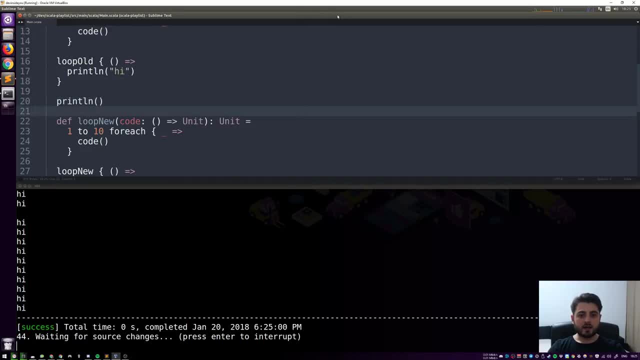 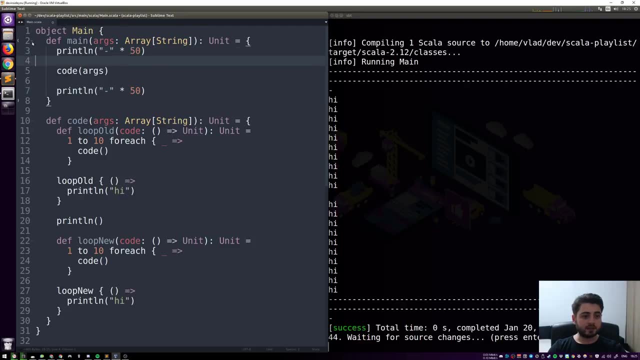 All right. So we have the first highest and the second highest, And in fact, let me actually do this and that right. So now we can see the whole code and now we just need only 50 hyphens. so let me collapse. 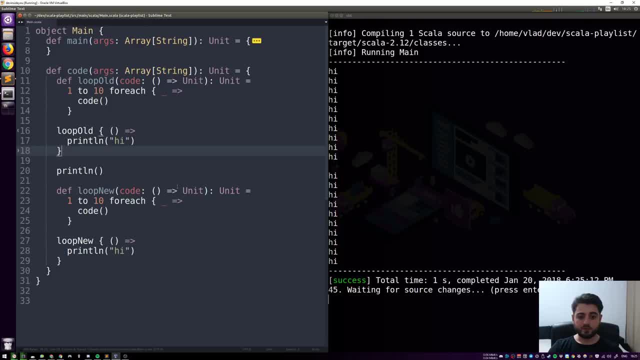 the main again. All right, So now you see both the old version and both the new version. okay, The next thing that I'm going to do is: you can do it almost mechanically, right? So I'm going to mark these parentheses, right. 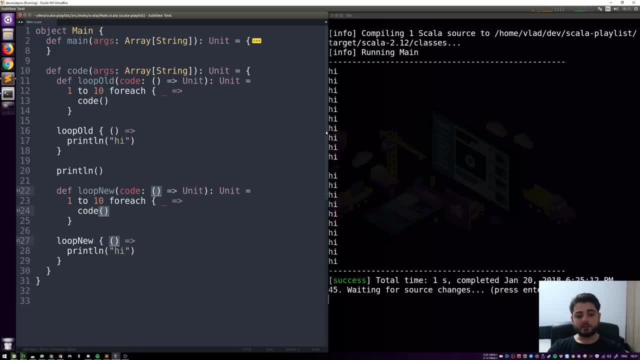 And I'm going to press control D and I'm going to press control D again. So in these three places we can just remove them, right, And in the very bottom one we can also remove the arrow. okay, And let me remove an S space over here, right? 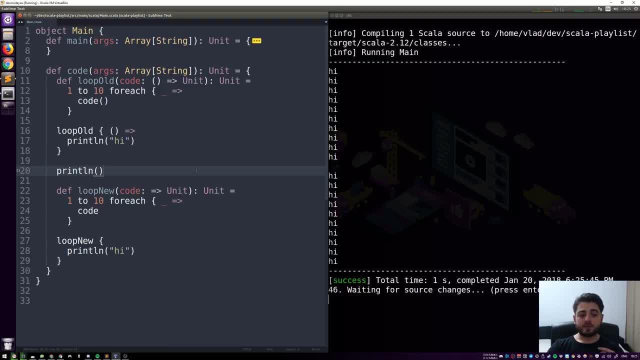 So these both pieces of code are equivalent. So, whenever you have a high auto function that receives another function as its argument, that does not receive anything, right. So the argument is that it receives a function. Okay, So the argument that this function that it's being passed to is a unit, right. 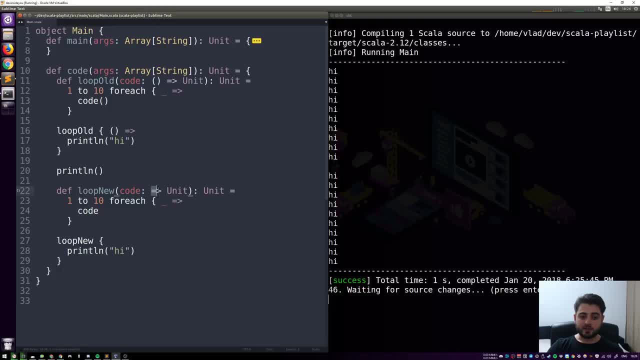 Then you can use this syntax, right? You can just leave the parentheses out, you just have an arrow and then the unit, okay, And then when you call it, you also don't use the parentheses, right? And you're doing all of that just so that your clients, right? 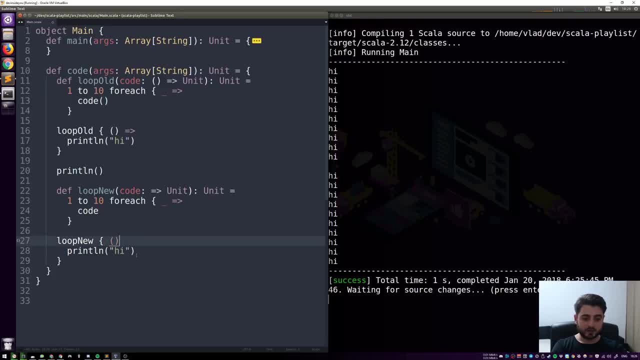 So that your clients don't have to write this thing, sorry, that thing, okay. So the client code looks actually kind of cool. Actually, let me rename loop new to just loop. Look at this code. It looks so beautiful. Just loop. print line high. 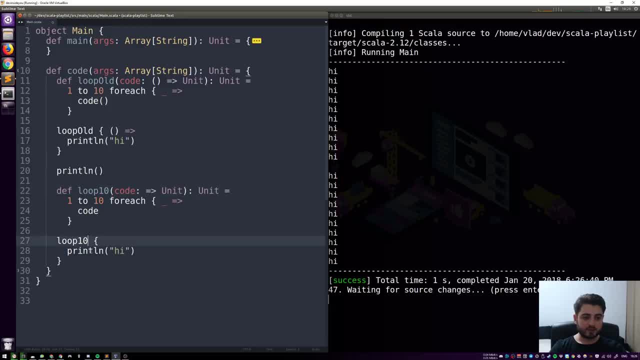 Actually, let me call this a loop 10, because it goes from 10, right, Loop, 10.. Loop 10, print line high. Two things you need to know about this. Whenever you don't have an argument like this, you're saying that you're passing an argument. 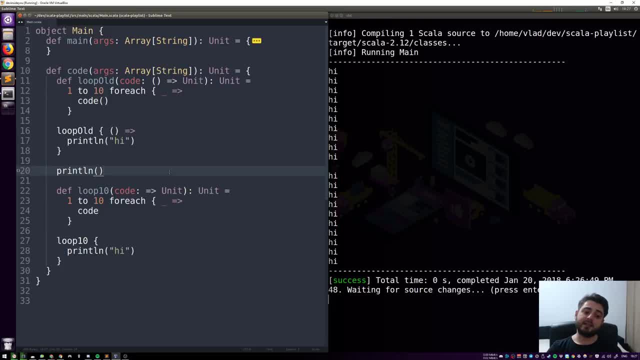 by value. And every time you do have this, you're saying that you pass this argument By name. It's just a convention, It's just being called by a call like that. There's nothing special about it, right? It's just. it's just syntax, right. 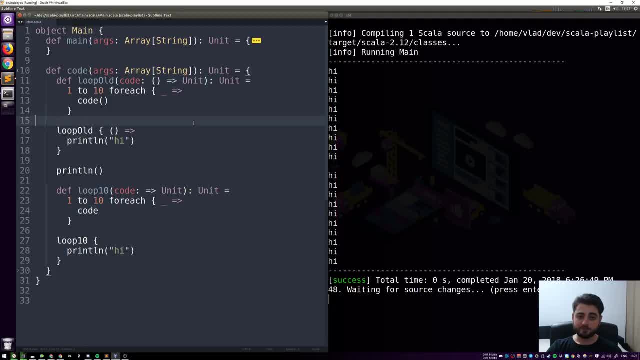 So whenever the compiler sees this, it will convert it into that, okay? The second thing you need to know about this- and we're going to discuss this a bit more, actually in quite quite a bit of detail, in the next video about inversion of control- 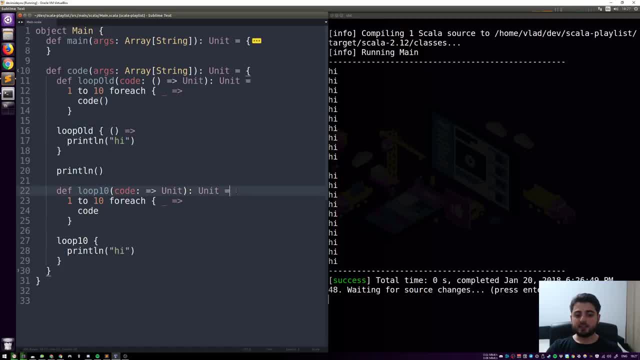 Notice that every higher order function is in charge now of this tiny function that you pass in, right? So it can decide, for example, not to call it at all, Or it can decide to call it twice, right? And if you have syntax like this, then you know that what you're passing in is a function. 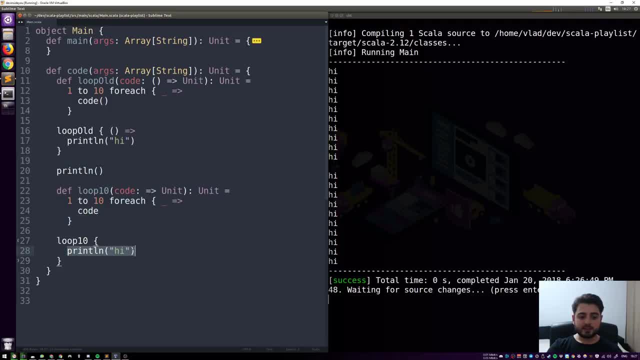 Over here. if you don't see the definition right, You don't really see over here that this will be wrapped into a function, right? You don't really see that this will be wrapped into something like this, right? So this is a bit more surprising. 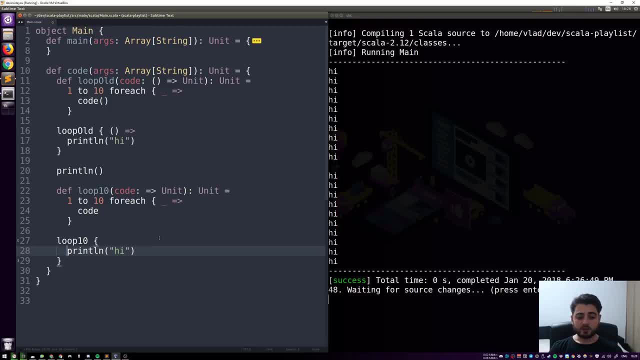 And when you gain more programming experience, you will understand that You don't really like that, right? So we don't really like libraries that surprise us, right? It's called the principle of least surprise, So always try to write your function in such a way that they will not surprise your callers. 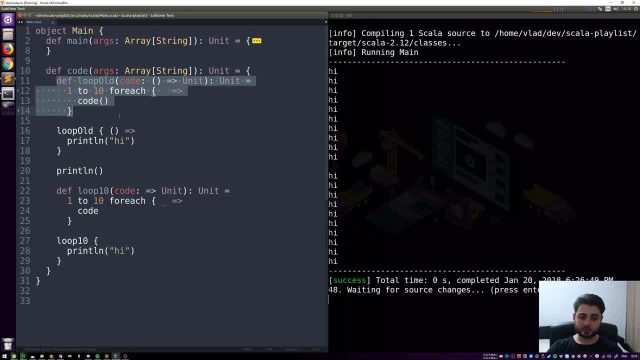 right. So this function, this syntax, is less surprising than this one, So apply it gently. Be very careful with it. All right, This is the end of this video, and I'm super glad that I finally made a video that is actually. 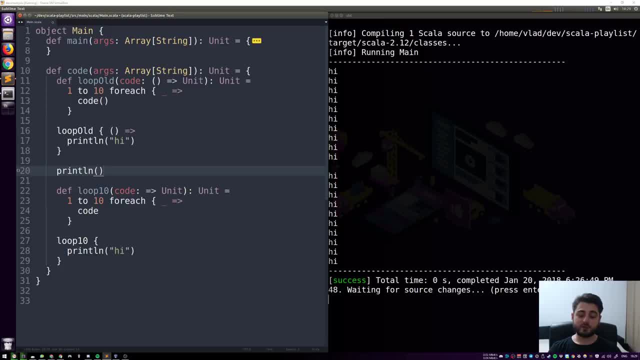 shorter, So Okay. Recording software shows me 46 minutes, So when I'm going to cut it, it should be like about half an hour. What you should know is that we're nowhere near done with high auto functions. Basically all the code that we're going to be writing from now on, we'll have them in. 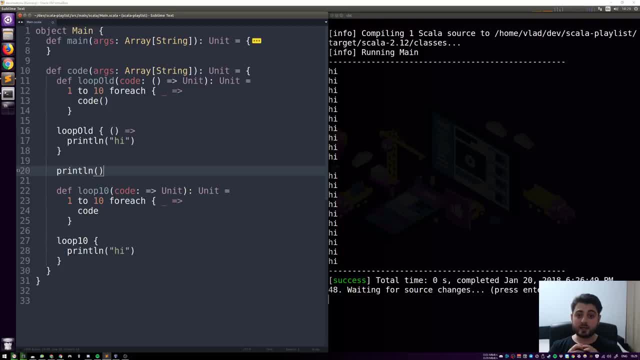 one way or the other, because they're just really, really useful and they're basically used everywhere. Sometimes you don't see them, Right, Okay, So I hope you liked this video, Like this if you did Subscribe, if you're new here, and see you next time.